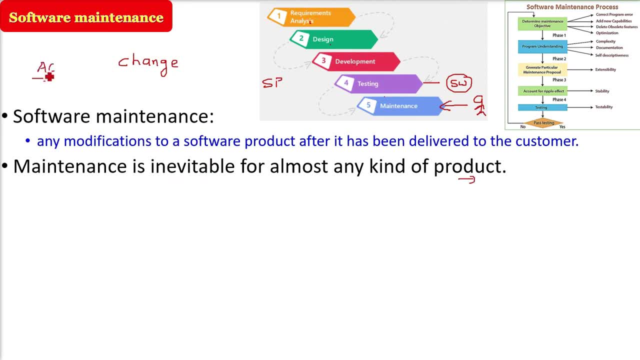 If you are having an air conditioner, You don't go for the servicing. the filter will get dust and it will be useless after some time. so maintenance is everywhere. most products need maintenance because they have the wear and tear like car now in the car, say, six to eight months you have 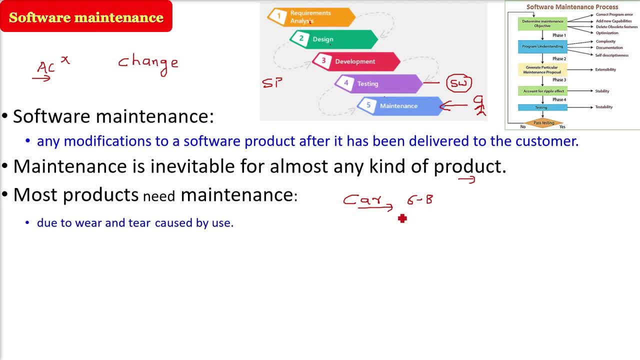 to get its serviced. there will be some wear and tear in the machinery. they basically the tires mainly, and these are the wear and tear mainly the product or hardware products. but software products they don't have this kind of problem, that is, they do not need maintenance on this type of count or 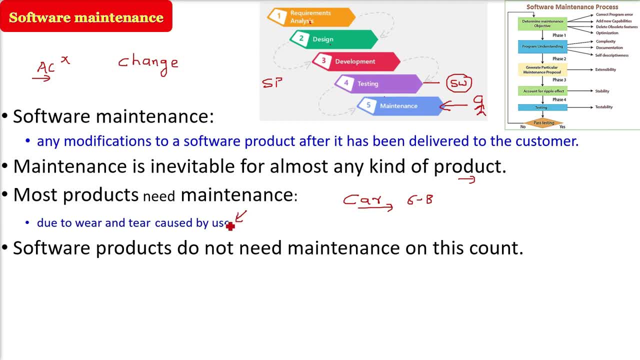 account, so there will not be a problem like this. software maintenance has something other to deal with many people. they think that if the bad software is created, you need a lot of maintenance. but this is absolutely wrong. the opposite is true. bad product- what do you do? you just throw it away. you don't maintain it. but 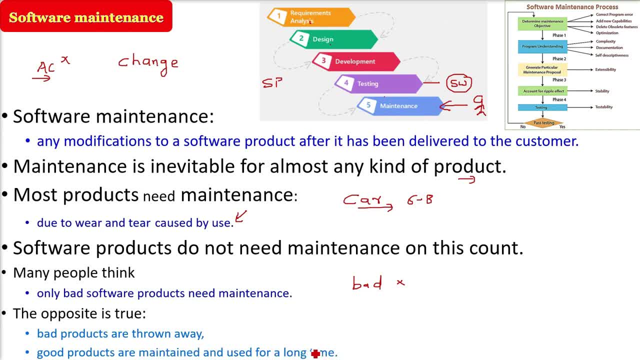 the good products, best products. they are maintained, they have longevity, so they are used for a long time. i'll give an example: see, when unix26 came, it was imported or implemented in assembly language. we have known about 885, 886, this microprocessor and language, etc. now, when C language came, the 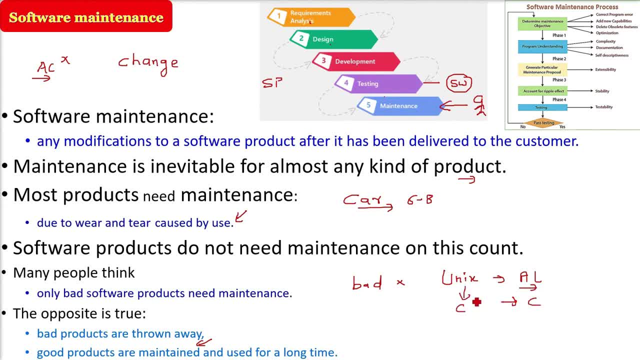 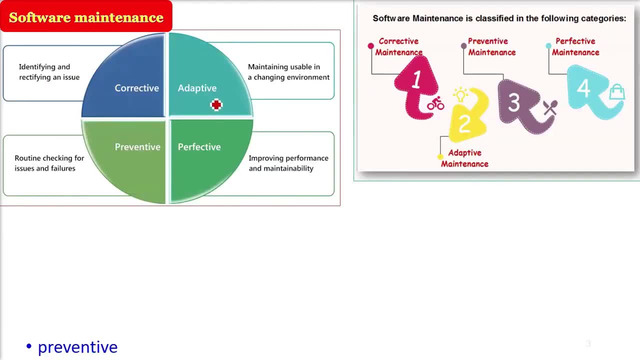 UNIX was rewritten in C language. Why? Because we wanted to keep working on UNIX, So we don't throw it away. This was a good product, So we need to maintain it because it is going for that. from the time it was being created till now, Software maintenance takes various 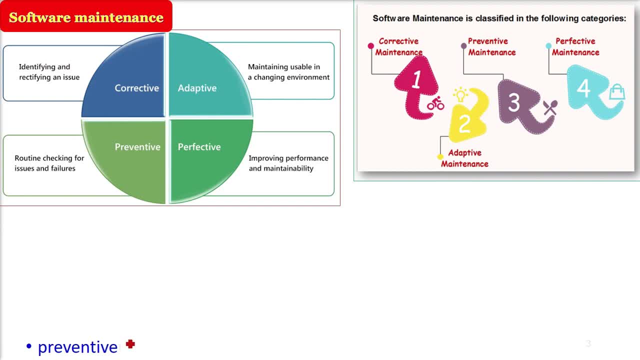 types. This can be done in four types: Preventive- I have written first because this is more related to the hardware stuff, But still, if you are being asked, you have to talk about all these in software maintenance as well. Software maintenance or keeping this software. 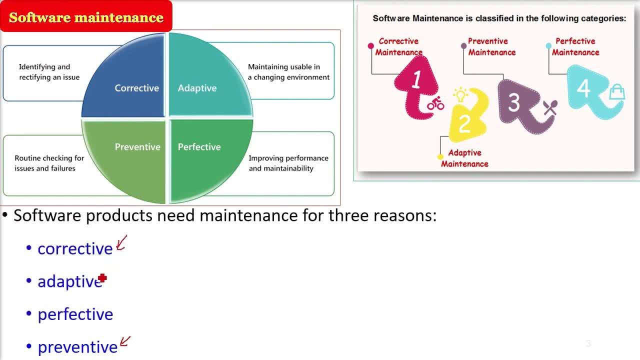 up to date. we need certain maintenance. First is corrective, adaptive, perfective and preventive. Corrective. adaptive, perfective, preventive, Preventive is the first kind of maintenance, because this is the fire cannot happen. Corrective is: fire happens then you. 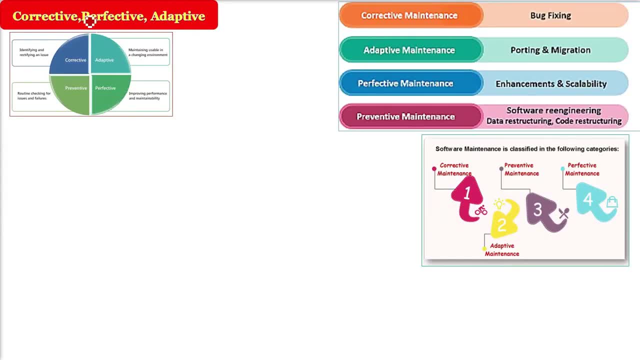 prevent it. So corrective maintenance, adaptive maintenance, perfective maintenance and preventive maintenance: these are the four types of the software maintenance. Corrective maintenance is all about bug fixing. So corrective means to correct it. That means something is wrong. If something is wrong, 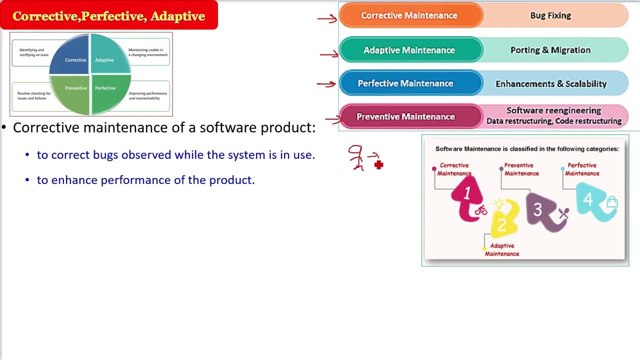 you need to correct it. If you deliver the software to the user now, user starts using it. Now user observes that, oh, there are certain problems here. So it will come back to you and say, oh, I am facing problem here. Now you fix the bugs. Then, for example, file transfer: 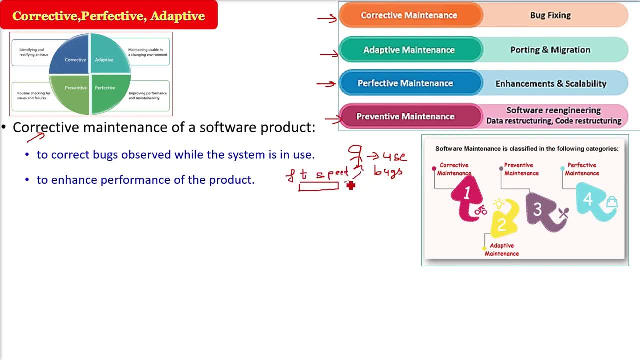 you have given him Now the speed you wanted. you are not getting it. You will again go back to the developer and then will say, oh, I need some enhancement on in the performance. So this is a kind of corrective maintenance. Well, it comes under the perfective also. 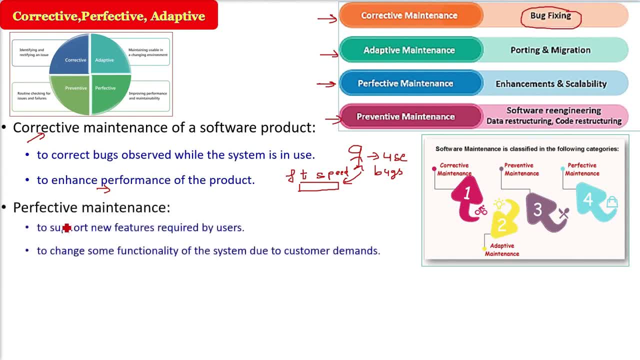 but these fun… These corrective maintenance is correctional maintenance, Corrective maintenance of the correction of certain things. What is perfective maintenance? Perfective maintenance is all about enhancements and scalability That is user is using. Now he wants oh, he say oh, these features. 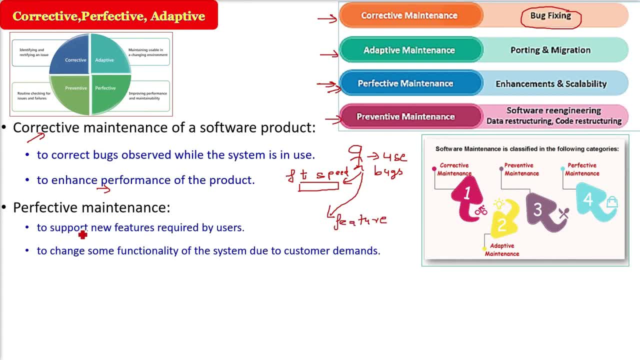 are missing. I need these features. Without this I will not be able to work. So perfective is the new features addition required by the user Or certain functionality he is using. he is saying no, it should be on the left, not the right, Or I need to change this functionality, So your 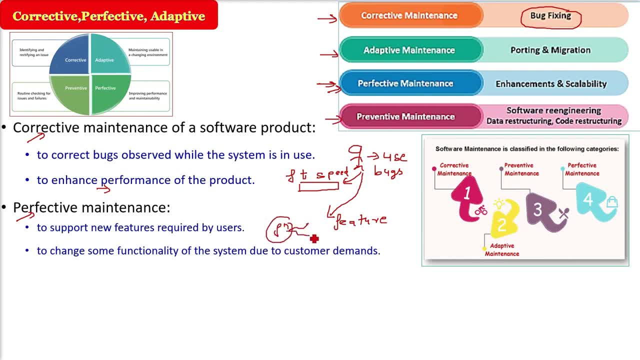 customer demands the change in the functionality and that when you do that is called as a perfective kind of maintenance. Okay, So it's all about enhancement and scalability in perfective maintenance. Then comes the adaptive maintenance, also called as porting and migration. So the 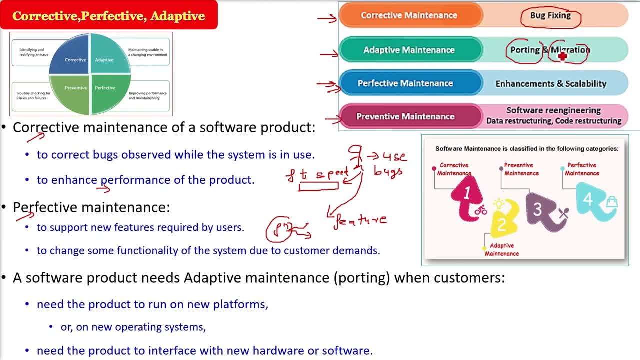 software product needs this porting or migration or adaptive maintenance When customer need the product to run. it should be on the left, So it should be on the right, So it should be on the left, So it should be on the right, So it should be on the right, So it should be on the right. 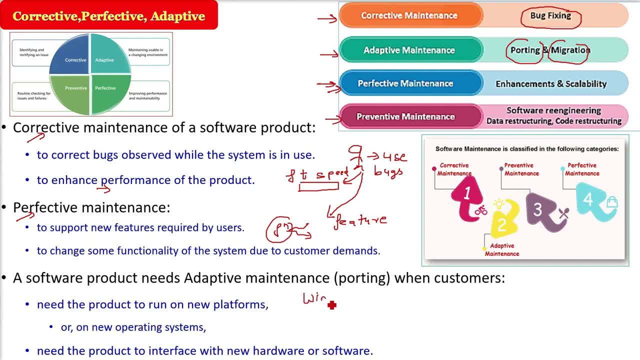 Run on new platform or a new operating system, For example Windows 10 you have. Now you have Windows 11.. You upgraded your system because it was free and the Microsoft was asking for it. Now certain software are not working on Windows 11.. So what do you do? You will go back to the. 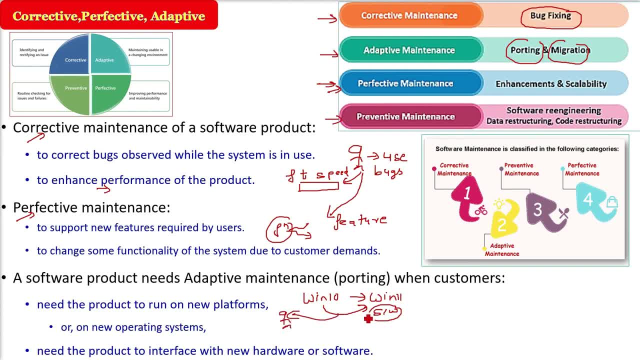 developer or the key company and you will say, oh, this software is not working. So the software team or the maintenance team, they have to do the adaptive maintenance so that this software work on Windows 11 as well. So new platform, new hardware, new configuration, new operating system, this kind of maintenance. 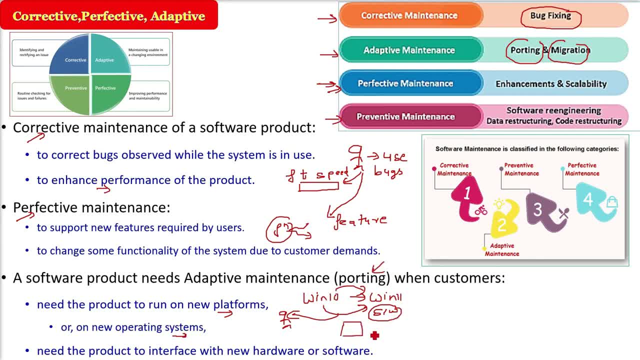 is adaptive. Now you have a product. Now you gave the interface for the serial port, serial port connection. Now somebody comes and says: no, no, no, I want the parallel port also. So these need some interfacing changes. This is adaptive maintenance And there is a preventive maintenance. 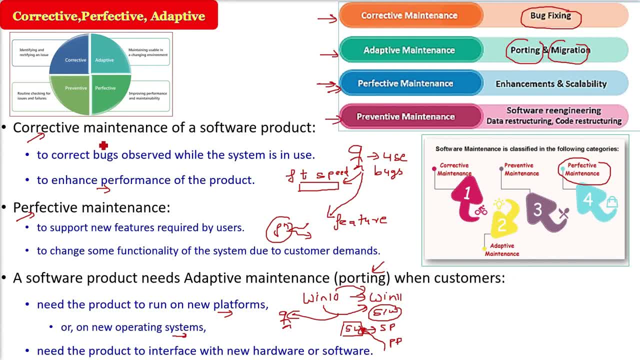 See, preventive maintenance is corrective. is fire has happened? Now you need to say firefight. But here make the code do something so that fire cannot even happen, cannot even occur. So the way you code, the way you design, you be aware that the maintenance activity should be as least as 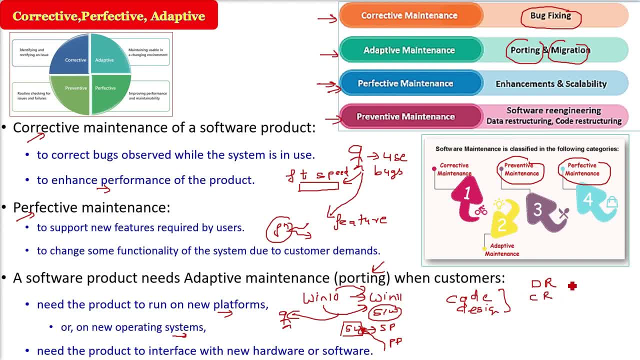 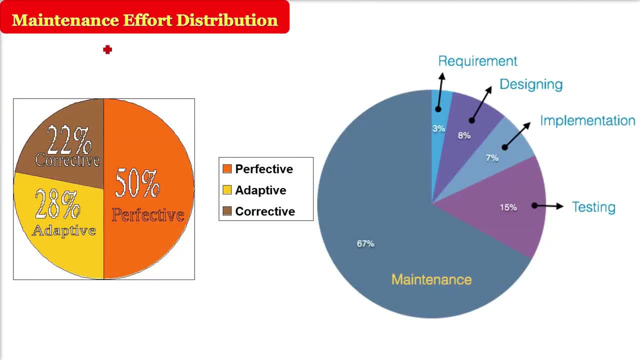 possible. So preventive maintenance is all about software re-engineering, data restructuring, code restructuring. The effort distribution with respect to maintenance. if you see different type of maintenance, 50% of the maintenance is perfective, 28% of the part is adaptive and 22% corrective maintenance effort is used. 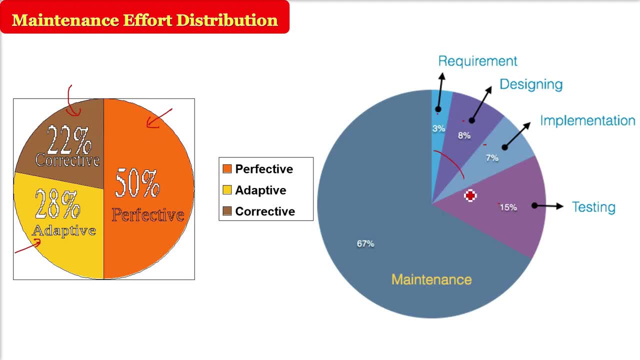 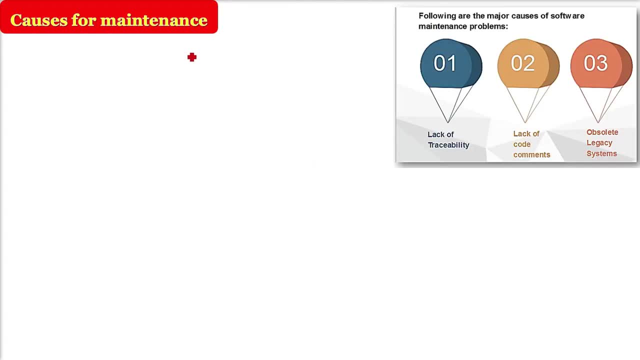 You see here: requirement, design, implementation, testing. What is this? part 67- almost part, is your maintenance part. What are the causes for maintenance? What are the several reasons? Why do we do the software maintenance? Why it is required. 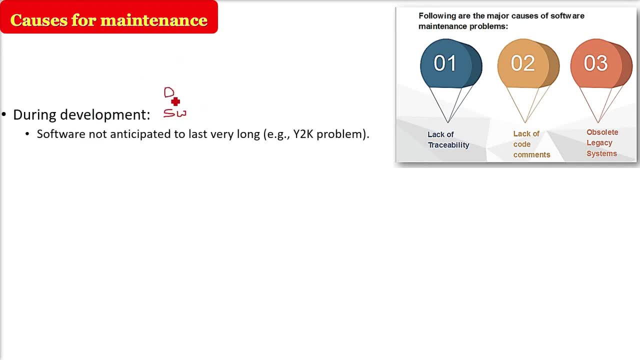 First thing is, while you're developing a software, that is, you have the requirement analyses, then you design it. On the basis of that design, this software is coded. Now the thing is that you are solving a particular problem of a user. 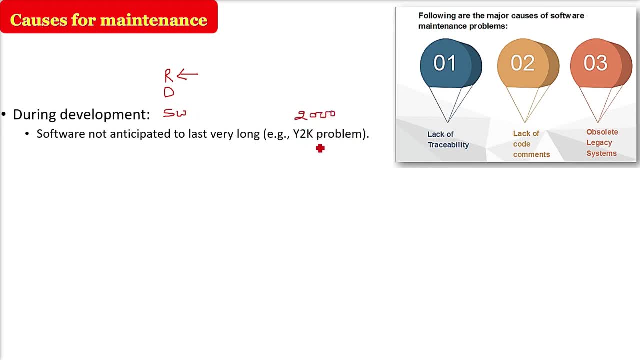 Now there is a problem which cannot be foreseen, Like Y2K problem. Never people have thought about it, And these kind of problems can be solved with regular information. not only Microsoft, inside the context of the service itself, I mean, that has something proposed according to the on the database. 45 people are all broadcast the dailyonomically, often 50 days a week. So you can, this is what, 35 days pretty much. for Neo, 25 days. you are using, obviously, the DI machine, out智 geez. Here is almost 30 days of the time this is going. 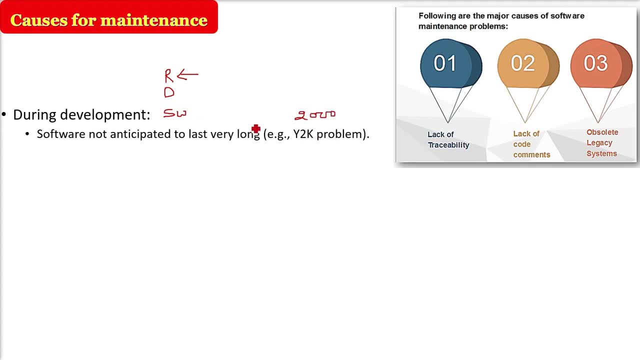 And these kind of problem can come anytime. So if you are not able to anticipate, then during development, when the product is already ready and it is being delivered and this problem comes up, then you need to do the maintenance Rate of hardware abolishance. 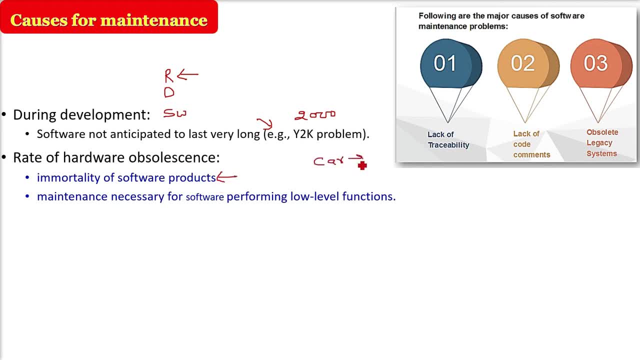 Software never dies. If you take a car- good car- 10,, 15, even 50 years, the car is going to die. Car is not immortal Because it is a hardware. It will succumb to its wear and tear. 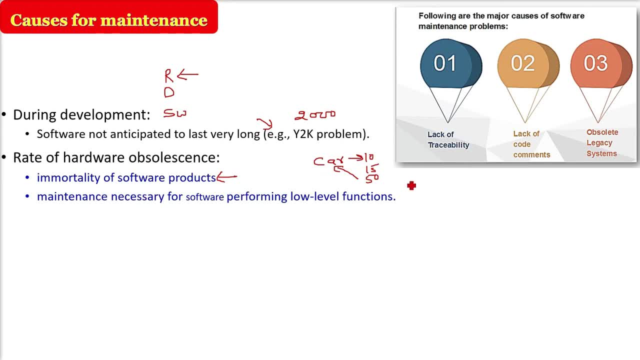 But software never dies. But maintenance is necessary for software performing lower level functions. That is the legacy software, The software which has been made. they have big, complex projects. Now it is being used widely. Before 1990, no one ever thought that everyone will be having mobile. 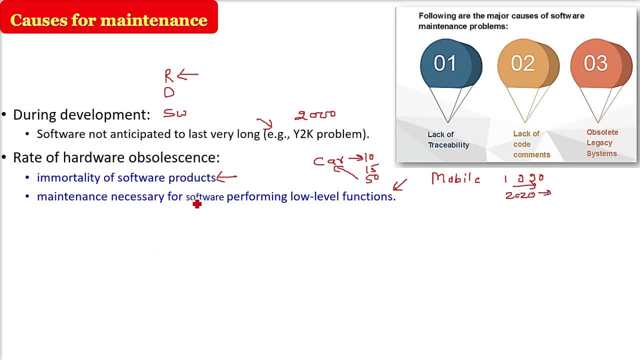 After 2020, now we can think that the kids are born With the mobile phones, with the cellular phones, with the smart phones. So you need to see here that the software needs to be updated, maintained every time. Whenever other software it works, they change. 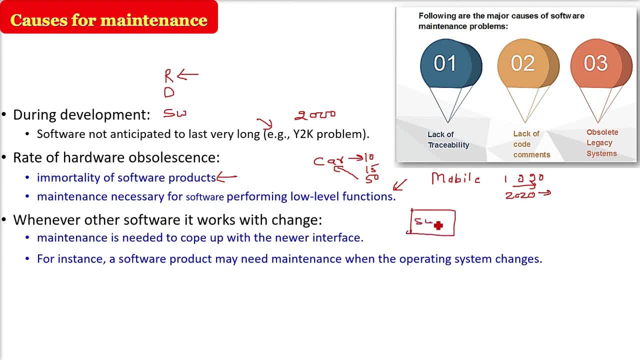 Okay, let me give you an example That your software is being delivered. Now you say USB, it will work with USB 2.0. Say USB 3.0, USB 4,, 5,, 6, 10, say 10 has come. 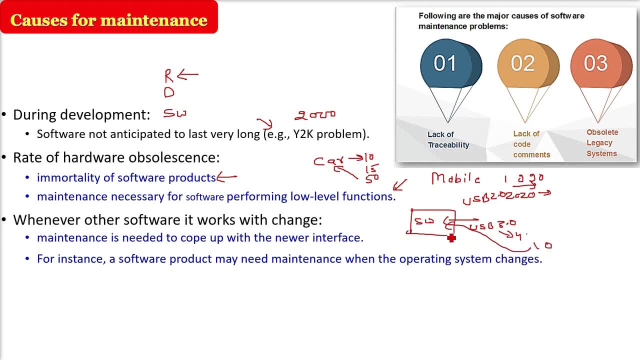 The speed is, say, 10 Gbps or 100 Gbps. Now it is your liability to change the software to adjust working with this new USB, See Windows 10, you are always going to Windows 11,. it is free update. 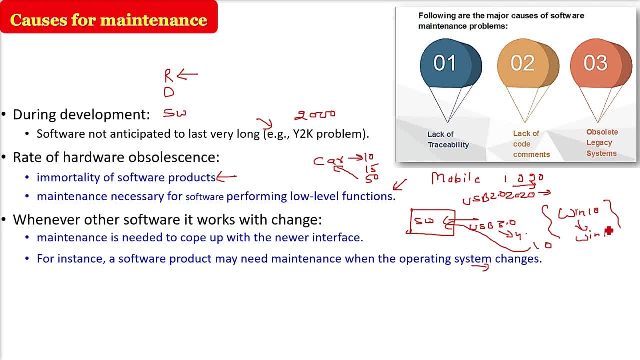 But what about? the software you are working is not working on Windows 11,. it was previously working on Windows 10.. The software product may need maintenance when the operating system changes Or user want existing software to run on a new platform, for example Windows 10 to Windows. 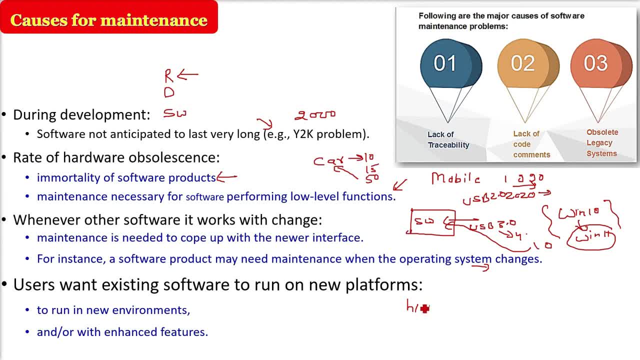 11 is a new platform, A new software, this new operating system, a new hardware is employed, a new configuration is employed. So if you have 10 functionality, the user can come. he says, oh, two more functionality evolved, or the government has changed some scheme or some numbers or interest rate, or 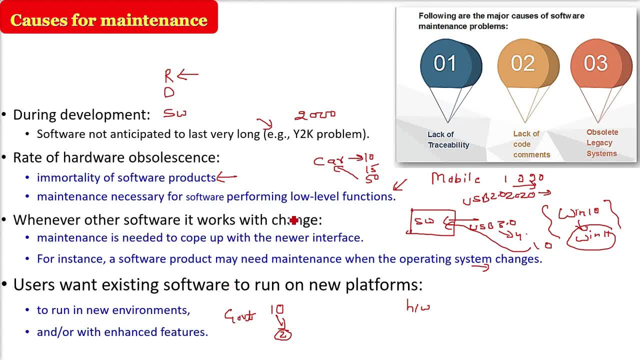 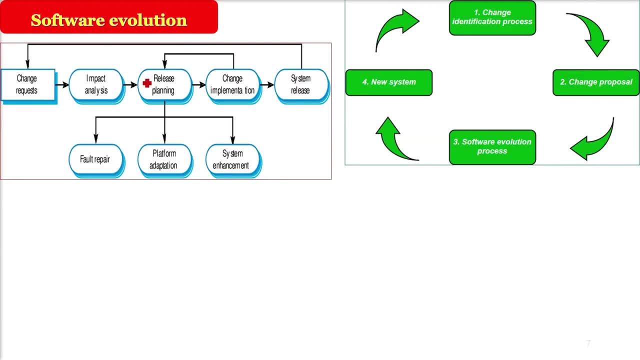 any other thing. So you need to enhance the feature. You need to do the maintenance, Like our human beings evolved from chimpanzees or monkeys, etc. We have evolved like that, So you need to do the maintenance, Like our human beings evolved from chimpanzees or monkeys, etc. 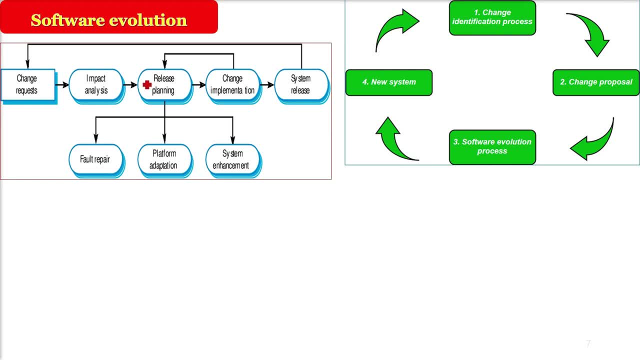 We have evolved like this and we are still evolving. The software is also like that. Software is evolving every time. The time it was conceived till now, it will be in the process of evolution. Every software product continue to evolve after its development. 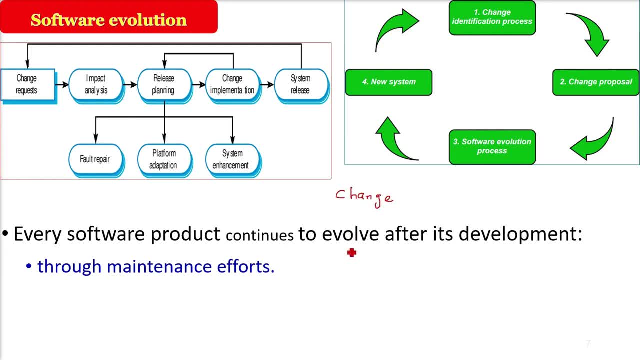 Change is the only thing which never changes, That is, we need to make it evolve through the maintenance efforts for the better. Evolving is making it better For the different environment, configuration, functionality, feature usage. So there will be some change proposal. 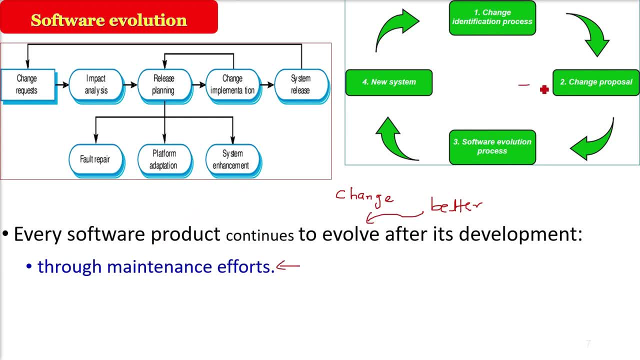 There will be some change request, always coming from the people or the end user, and you need to change it, make it better, Larger software product the complex, which are being used by numerous people Now. this software was made with immense amount of money. 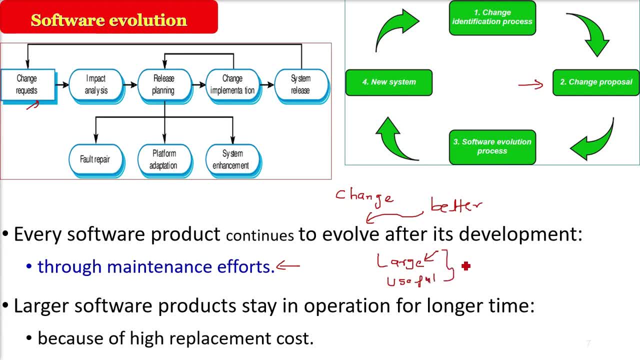 Now it not be viable or feasible To replace it entirely. it will cost more, So better is to maintain it, Like artificial intelligence, or now the Google products have AI involved, But 5-10 years back they were not having that. still they were popular. 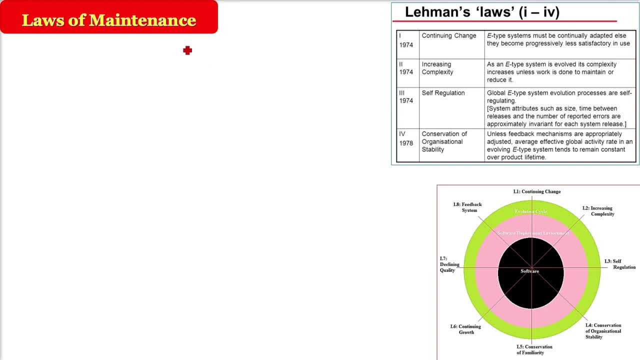 Laws of maintenance. So there are certain laws, there are rules for the software maintenance, and what are these maintenance? before that? There will be lot of old software. The software which is made today will be old tomorrow, So there will always be a lot of old software that will need maintenance. 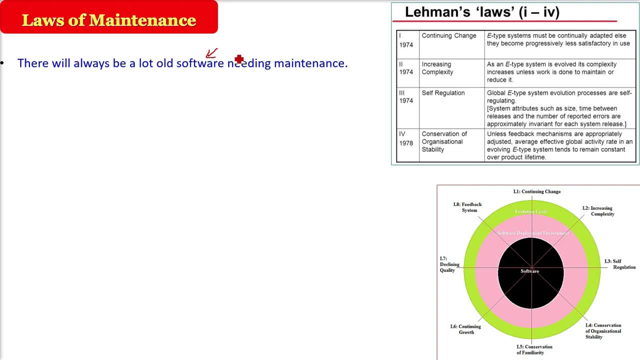 The user will want. the user will change, the technology will change, the thought process will change. So the software has to change And if you have made a good product, it will be maintained, Because the bad product will simply be thrown away in the dustbin. 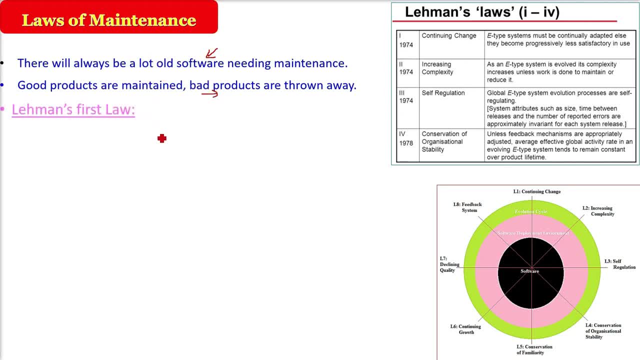 So there are certain laws of maintenance. The first one, This is Lehman's first law. The first law says: see, these laws are very common sense law, But since he has predicted and presented their laws, the first law is: software product must. 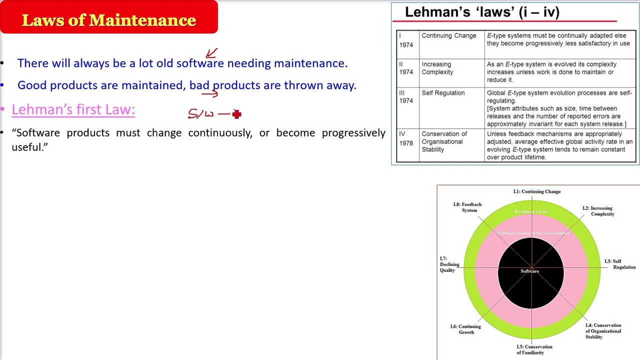 change continuously. If they are not changing continuously, they will be useless. That is, they are useful only when the software products are changing continuously, evolving, modifying continuously and becoming progressively useful. Otherwise they are useless. The second law of Lehman says: when software is maintained, its structure degrades and it 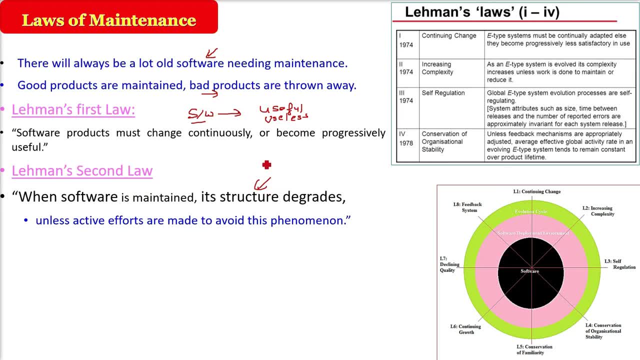 always happens. You know the regression testing. why do we do it? If you hire a maintenance guy and he is not able to maintain properly, one part is having a problem bug. he tries to fix it and he creates 10 more bugs. 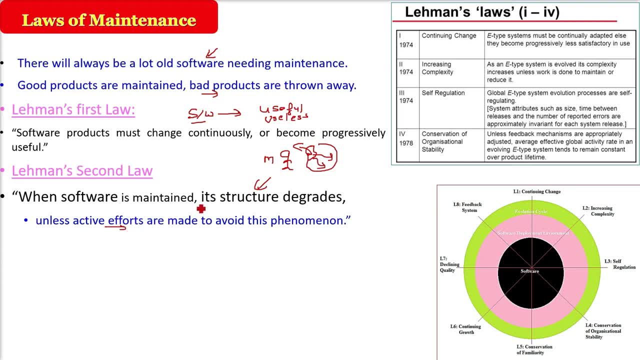 For that you need to put a lot of effort in the maintenance phenomena Because you really want to maintain it, You really want to avoid this kind of regression or propagating or bug say network strategy. Then the Lehman's third law: Over a program's lifetime its rate of development is approximately constant. 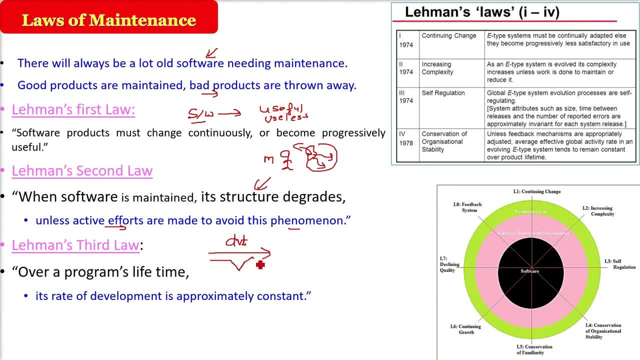 There is no peak, there is no trough. Sometimes you are developing a lot, sometimes you are not developing. sometimes you are changing the software, sometimes you are not modifying it. So, right from the requirement, design, coding, testing, deployment, development, development. 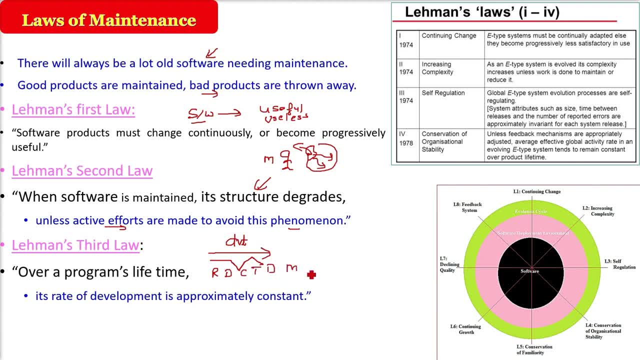 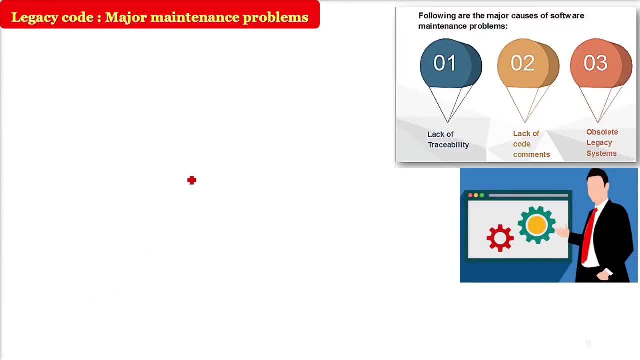 development. That is the third law, The software development and maintenance. the software development rate of development with time remains constant. Legacy code: There are major maintenance problems. So what software, what system has already been made years ago and what are the major? 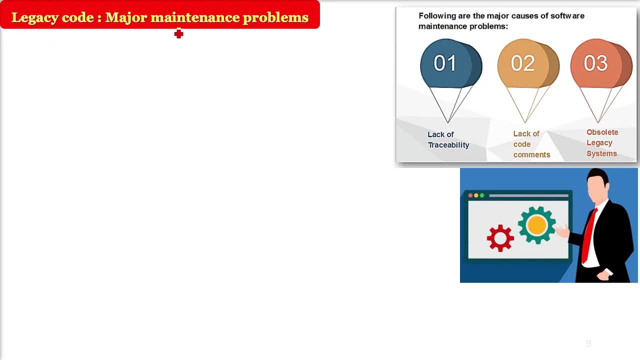 maintenance problems we perceive or we encounter. if, first of all, the maintenance engineer, When he is a maintenance engineer, When he is a maintenance engineer, When he is a maintenance engineer, He sees this code, He finds something. First is the unstructured code. 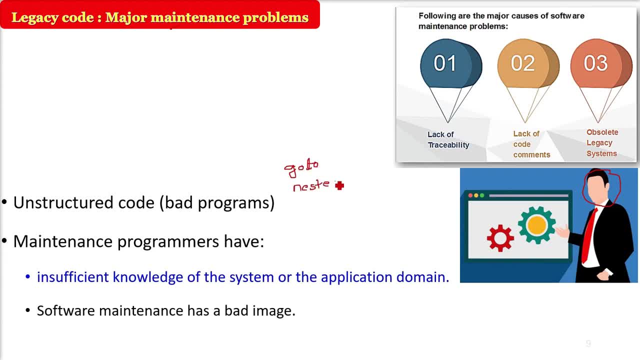 You have bad programs. You have written goto, You have lot of nested, if else multiple, if else Ruby construct. You have big procedures like thousand, two thousand, five thousand, hundred, thousand line. So that means bad program. You have very, very high coupling and low cohesion. 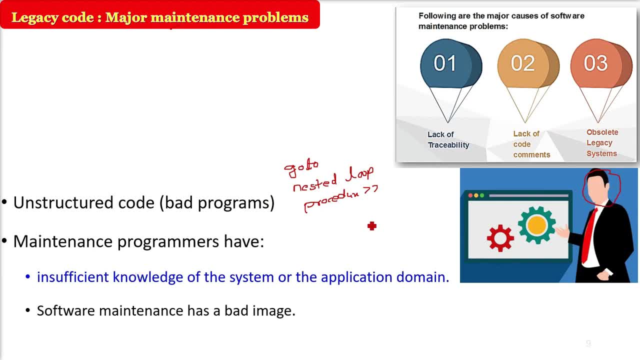 So this maintenance programmers, servers. they might not have the knowledge or they have insufficient knowledge for the maintenance of this sort of a system, that is, he might not be having enough knowledge of the application domain. So software maintenance. as the name has grown, evolved, it has taken a bad name. 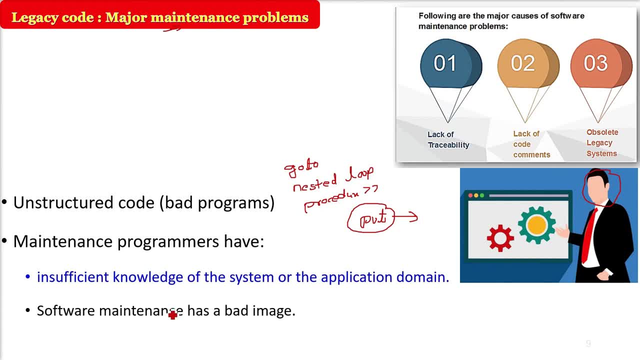 Maintenance means you have a problem, then only you do the maintenance. The software maintenance is like having a bad image Sometimes. a good software is always a good software means you have good work products like the software product, but not only the code or the source code. you have the documents. 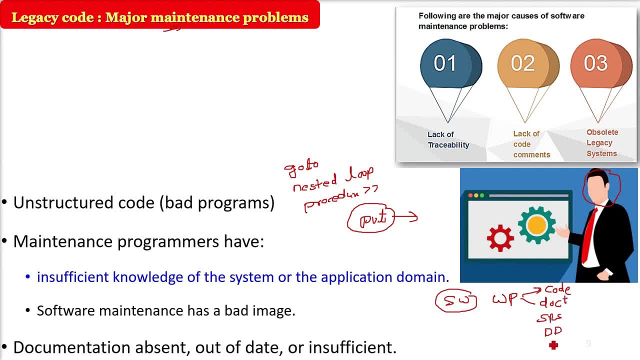 as well, like the software requirement specification design document, with all the UMLs test plan, user manual, the installation guide, the compilation guide. there are so many documents which will, which will help the coder and the maintainer, But sometimes the document is absent, out of date or even inside the system. 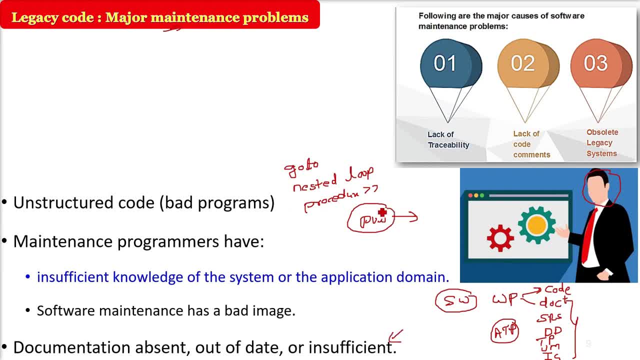 Insufficient for anybody to actually understand. even if a very good maintenance guy you have hired, you will not be able to find anything to do. So I will show you at these all. I'm just giving you a hint here. there is goto here. 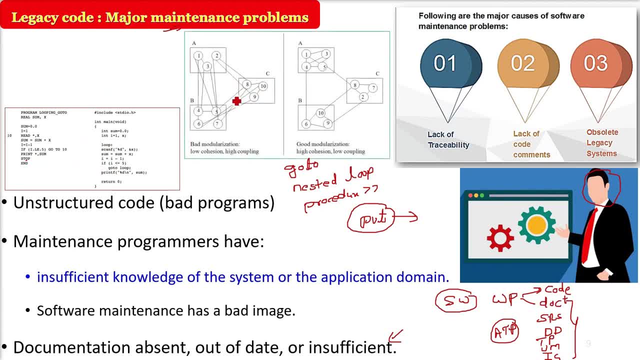 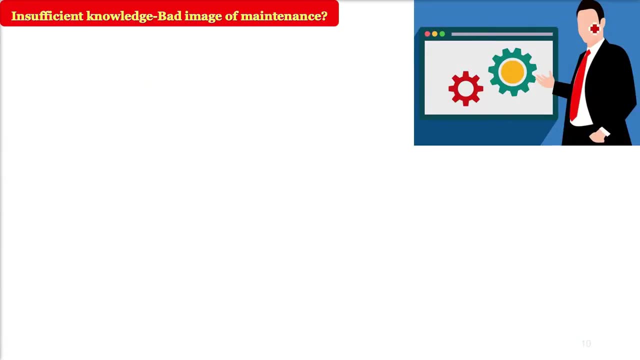 this is very bad: modularization, low cohesion, high coupling. we are always going for high cohesion and low coupling And then we have nested, if else the person is going to fall through his mind when he sees it. Insufficient knowledge, Bad image of maintenance. 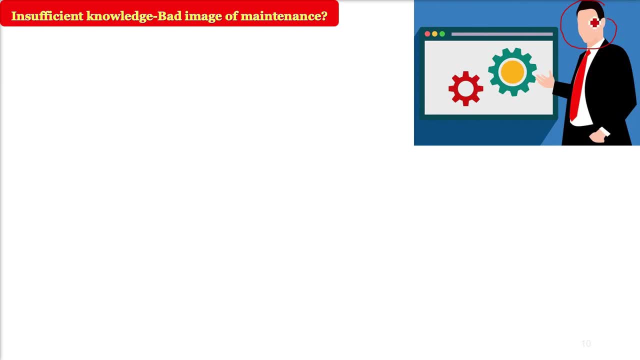 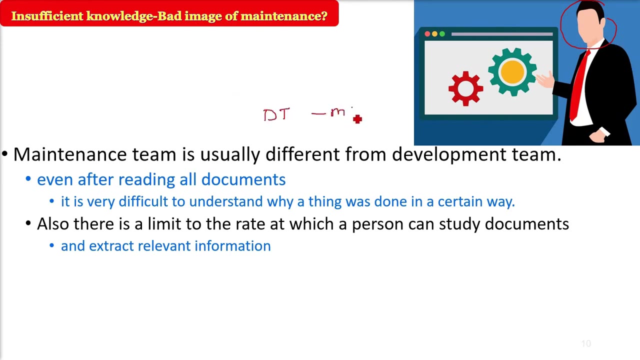 That is, the maintenance guy may not be good, or if he is good, then the software he is going to maintain is not good in terms of the documentation, in terms of the content he needs to understand. So the maintenance team is usually different from the development team- not always, but 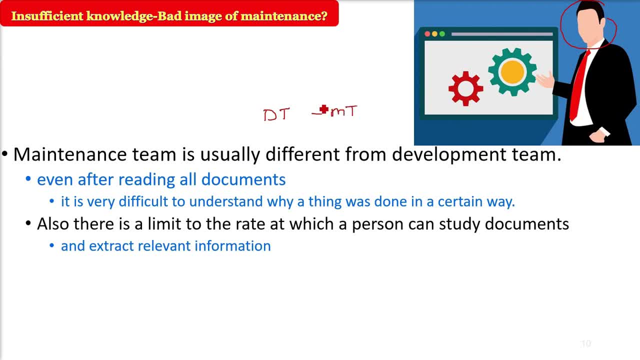 most of the time You will always see: oh, the guy has gone to America why he is maintaining the software. He has gone to the United States Why He is going to the offshore to maintain the software. So there is a different theme. 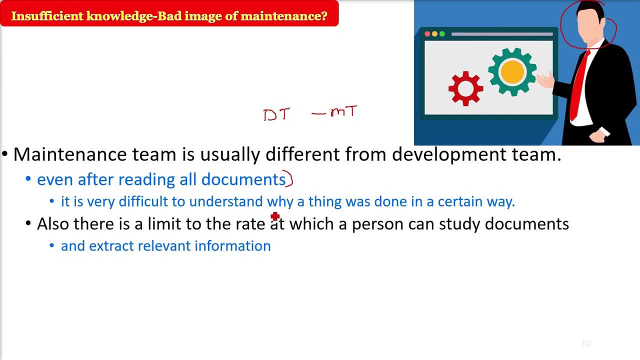 Even after reading all the documents, sometimes it is very difficult to understand that thing is done in which way. in certain way, Because they have not created the software. they are just trying to understand the software. What was the intent of that people, those people who have actually made it? 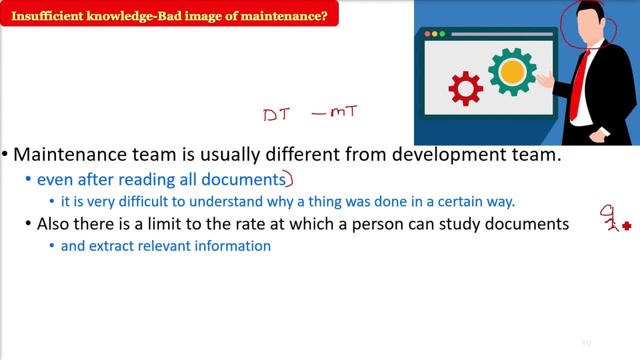 There is one more thing. it is human say limitation. If I read a book, I am talking about myself. I start reading, I just sleep. So if you are being provided those documents and if you start reading, may not be possible. 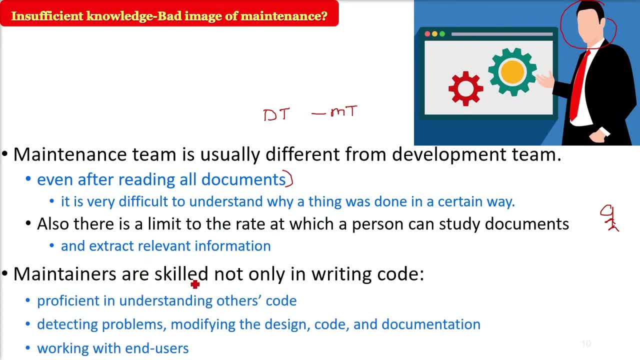 you will extract each and every information. So maintainers may be very good in writing code, they are very good at programming. But problem is they may not be good in understanding some code which is written even by other person. You can write code, understand it, may make any code. how about knowing the code from? 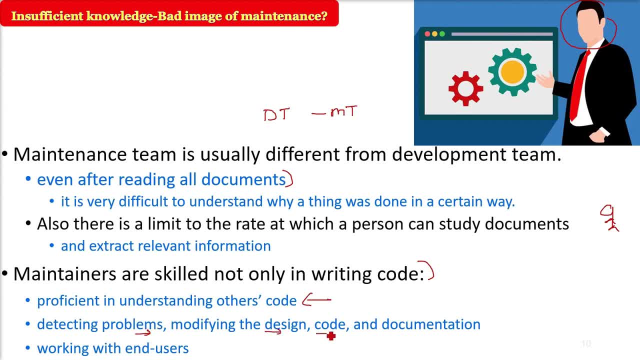 others, Parenting the problem where it is the bugs, modifying the design code or documentation, is again very difficult by a second person. And the most important part, which comes as an interpersonal skill, working with the end user, trying to understand, trying to solve. this cannot be a cup of tea for everyone. 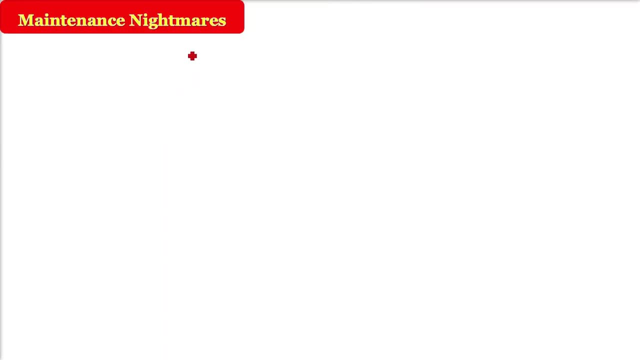 So working with end user is also a hurdle. Maintenance nightmares: These are the things which will always be there And giving nightmares to the maintainers. First is the use of Gotoos. This is a simple code, you see, it is written in basic. one more code: it is C, so you have. 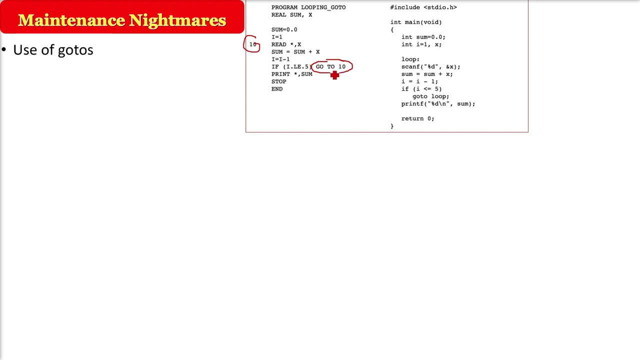 a Goto. Now, previously, when it came Goto, everyone was saying, oh my god, what a looping construct. oh, this has solved a lot of problem, But it has created a lot of problem. This is a Goto. It just shifts the program control to anywhere. 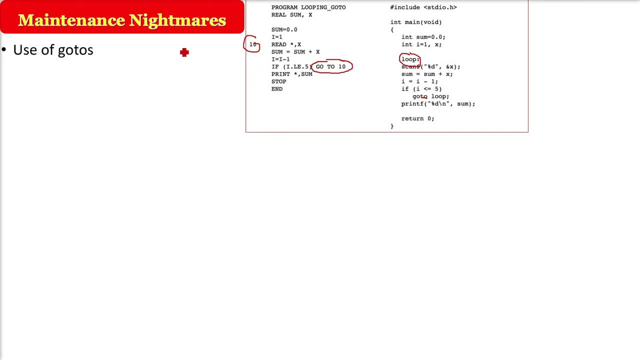 Even a big aircraft succumbs to it. Even a big aircraft succumbs to it. Even a big aircraft succumbs to this problem And many people died. That is why in MISRA standard they say no Goto at all. Then the procedures. 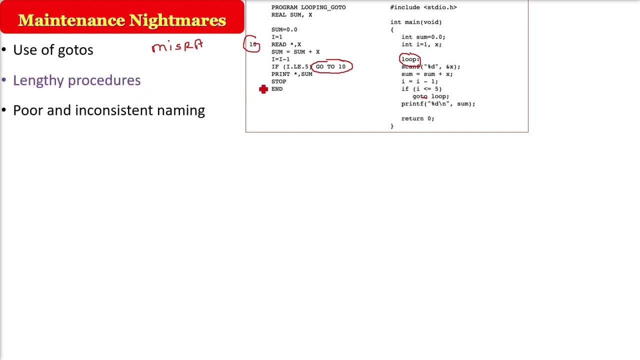 We are thrilled to write long, long code. oh, I have written this much of code, But they are lacking the procedure. What about modernization? What about the cohesion? So procedure should be small, should be maintainable, should be testable. 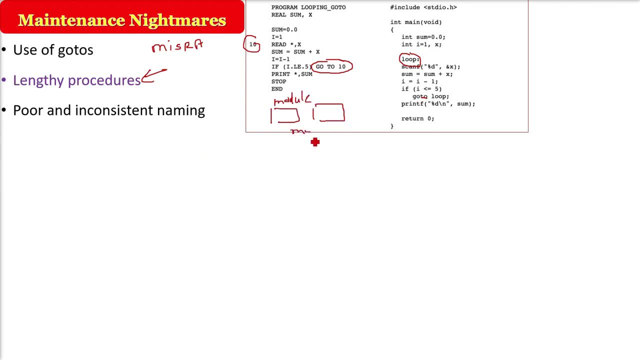 Poor and inconsistent naming. Now you just write name like you make your emails uglier, mycracking insta story like this: This is the name of your variable And we have seen this kind of names. Function is of add. 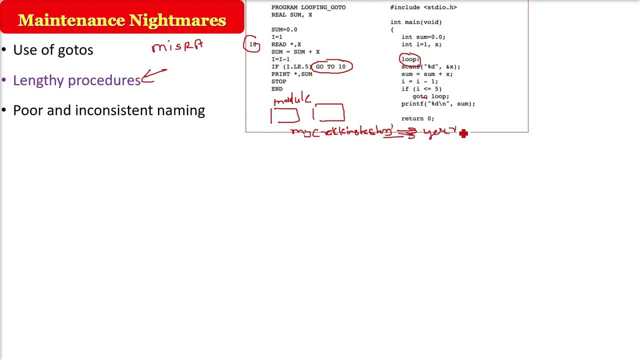 Now you are writing your, say your FB peak. this kind of name I use normally. The poor and inconsistent naming is one of the nightmare: Poor module structure, Module structure and email. This is the problem, And even the interdependence network of the modules. 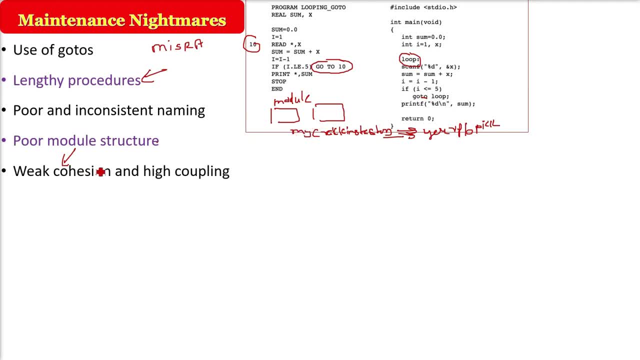 These are the key problem in designing So weak cohesion and high coupling. See when you are making modules. See here you have different modules and they have weak cohesion. They are not doing a single work. They are actually taking work from different module: giving them, taking them. 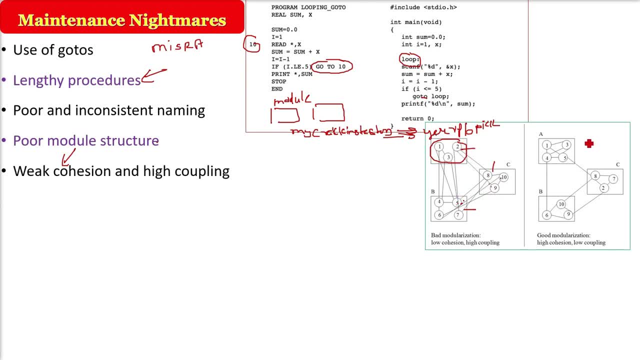 So there is high coupling also. But here A good modularization, good program structure or module structure means a module should do what it was intended to do, single work, That is. we need high cohesion. High cohesion we want. Normally we find weak cohesion. 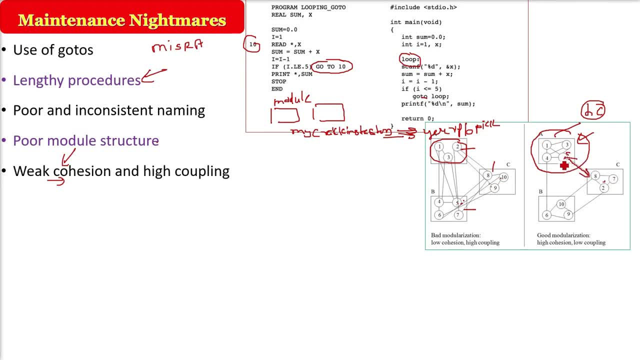 When multiple modules are interacting with each other, we need low or least possible interaction. That is called the low coupling. But we find high coupling Deeply nested, Deeply nested, Deeply nested Nested conditional loops. We have lot of statement. 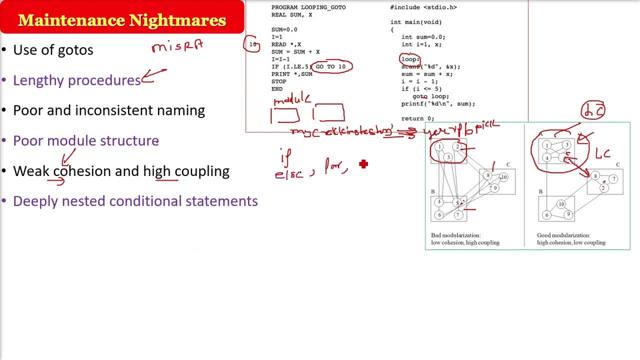 Conditional statement, If else For While Do, while Good is almost finished now. So these are there. When we program, we tend to put all our logic mind brain in making this kind of structure. What will happen? The mind will fall like this: 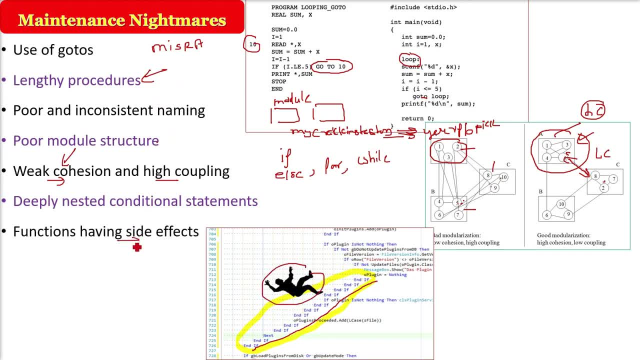 The person is falling here. Functions having side effects: We create functions which are meant for good, Made for good, But we are actually creating side effects. We create function which are made for good, We create function which are meant for good side effects. they are actually creating trouble in other codes, other functions. 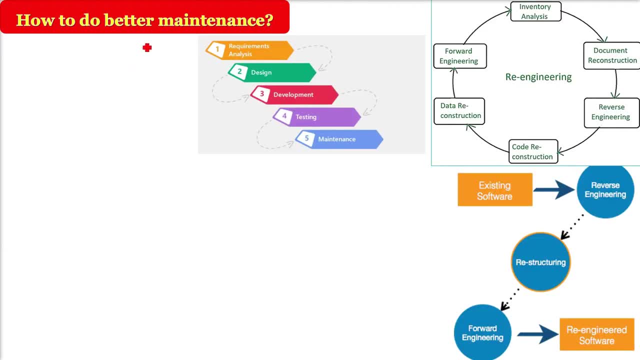 how to do better maintenance. software maintenance. this is the last phase in the software development lifecycle, but it is the most important phase. so how do we do it? we need to know the program first. either it is a software or a system. the understanding is the key. then we can do the re-engineering, the 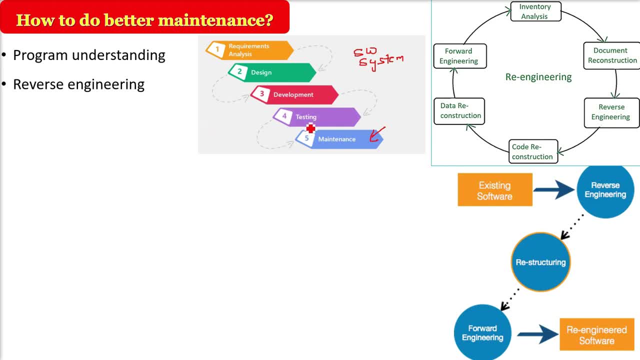 reverse engineering and the forward engineering. they both are combined and they are called as the re-engineering. so we have to find out in this reverse engineering, the design. so we need to recover the design from the code and the specification from the design. then the re-engineering, as I said, was going back. 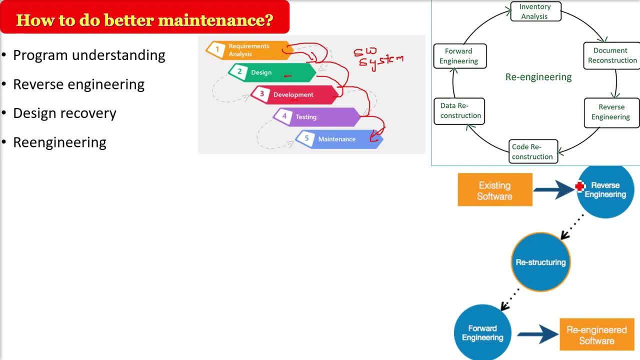 reverse engineering and then going forward. that is the forward engineering. So these are the steps to maintain, to do the maintenance properly if the project is complex, big and if it costs more to actually replace the software, So it's better to maintain. There are different maintenance. 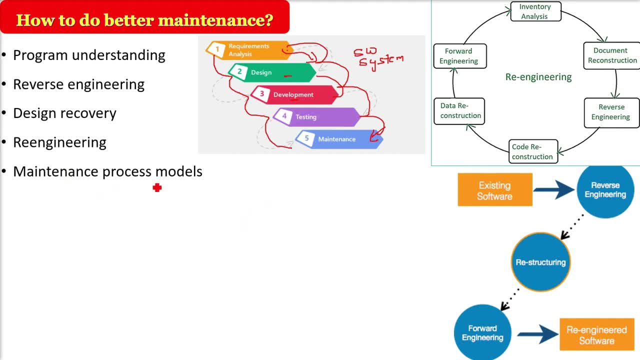 process models, depending upon the complexity, the cost and various other factors of a software under question. So the maintenance activities. we can divide these maintenance activities into two parts. They both are done, but one is productive, the other is non-productive. Non-productive means no work product is coming out of it. That is, this is the time. 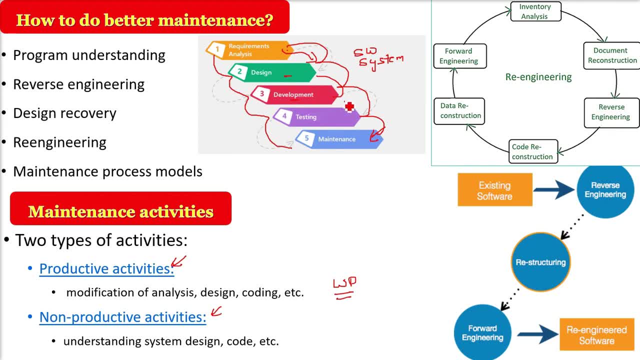 a maintenance guy or a maintainer. he would like to understand. he would try to understand the design, the code and of course the intricacy, how the software was made. This is the understanding part, So it will not produce any kind of result, But the productive activities in maintenance. 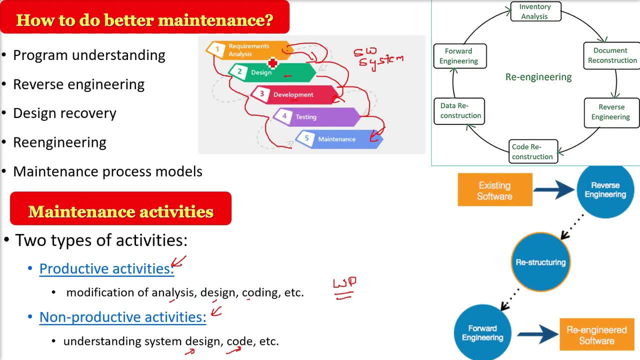 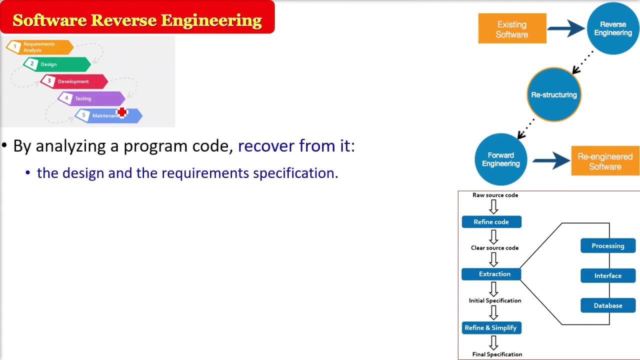 is analysis, design and coding modification. That is, you are actually trying to learn the code, trying to come up with the design and then the requirement, specifications, Reverse engineering in software. So how to do this? See, if you are in a car and if you use the 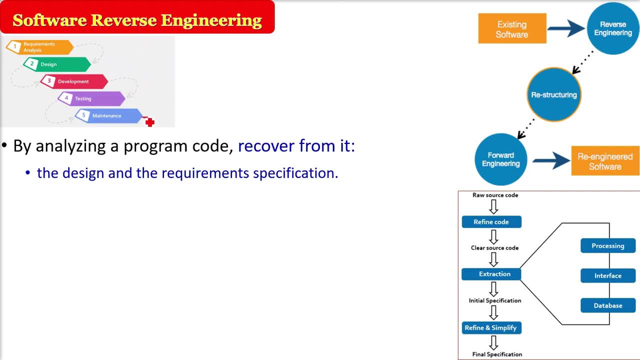 reverse gear, your car goes backward. Same thing here. You are at maintenance right now. Now you are only having the source code. Now, sometimes you may have the additional document or information, but you are analyzing the program code and you are only having the source code. So this is the. 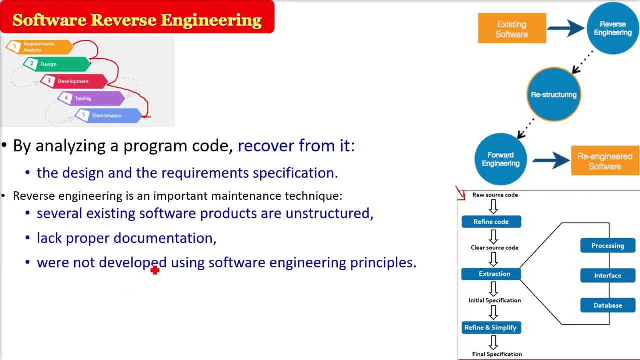 process of having a software and then recovering from it the design and finally the requirement specification. So reverse engineering is a very important maintenance technique. Why? Because there are certain software which are unstructured. They don't have proper documentation. Documentation is one of the work product of any kind of deliverable of software And they, these software, were not. 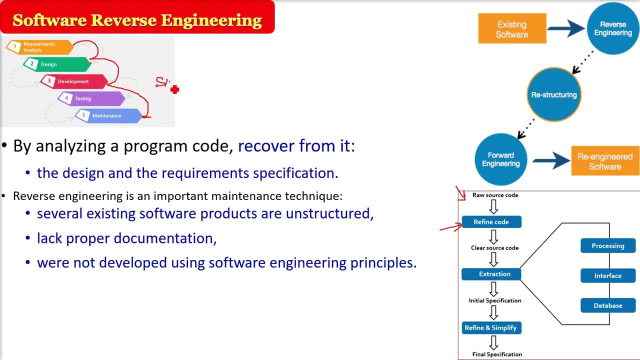 developed using proper software engineering principles, Not proper design, not proper coded. so the first we need to do the cosmetic changes. like your face, you want to go to the party. you will put some cream and some powder like the talcum powder, etc. so you want to improve. 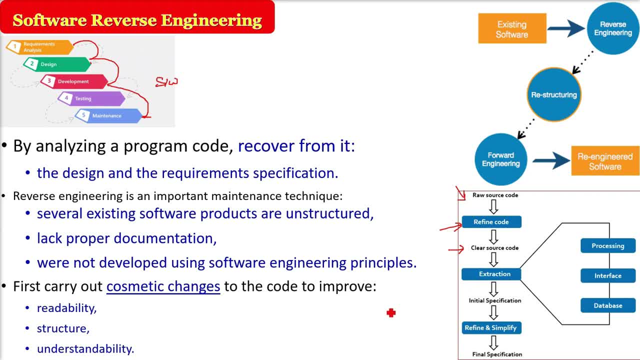 the readability. you want to improve the structure and the understandability first of all, before you can actually try to learn the code and come up with a design of this code. and finally, the requirement specification. so we need to find out first, clear the code, then try to extract the. 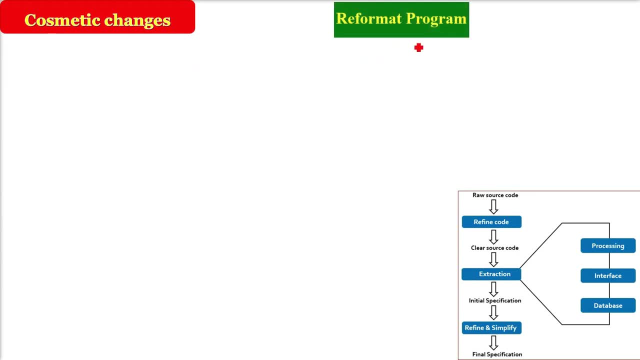 design and then the specification, so the cosmetic changes. the first is that you have a code with you. you need to reformat the program, the formatting to be done properly and most of the time, the maintenance, the involves the changing of the names. it can be variable name, it can be data structure name. 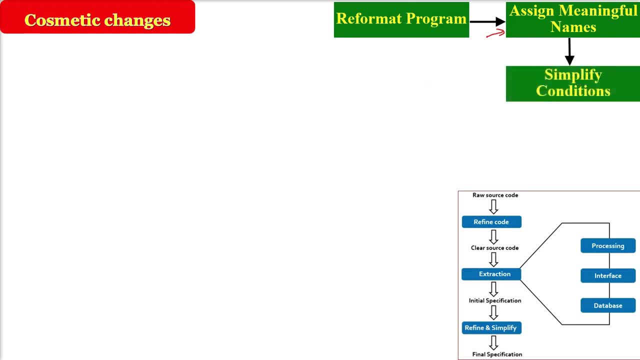 even it can be database name, so assign meaningful names. and then there are certain logical conditions. there are certain conditional conditions, so these are all. if i have two boils, and logical and, and or and not, and all these are used, then you need to simplify this condition and if at all there is replay, this go to just replace this, go to, that is, you are to you are. 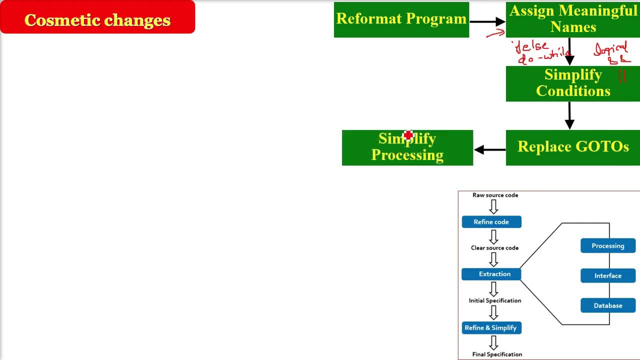 just trying to do the cosmetic changes for the program to look beautiful, to be understandable. so you need to reformat the program, that is, the layout should be made neat and you, as i said, you have to give meaningful names to the variables, to the data structure, to the function. names should correspond. 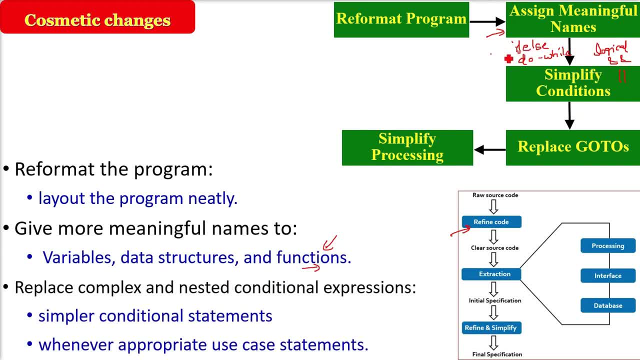 to what the function is doing. then there are complex, one by one, nested, looped, multiple nested conditional expressions. you need to simply uh, uh, sería to change it to your fancy. you know standard. You need to simplify these conditional statements and, whenever possible, rather than having 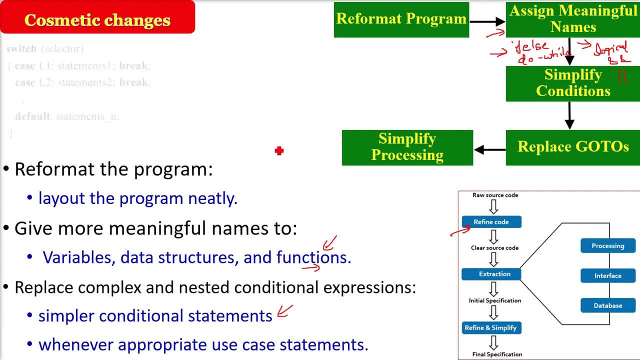 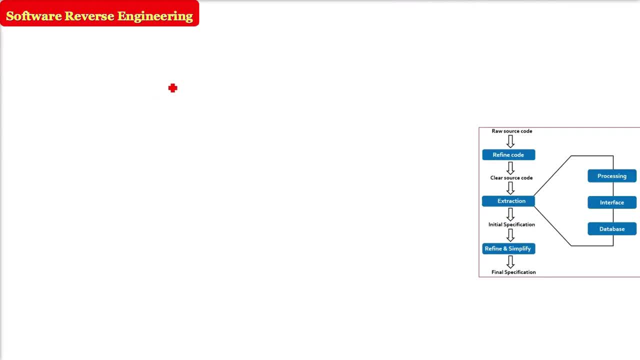 multiple if-elses, you can use case statement. This is the switch case statement. If your programming language allows, use this switch case construct. So in this reverse engineering, what you want to do, You want to first extract the design. 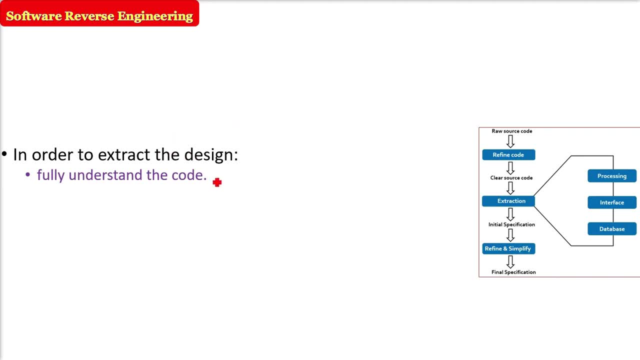 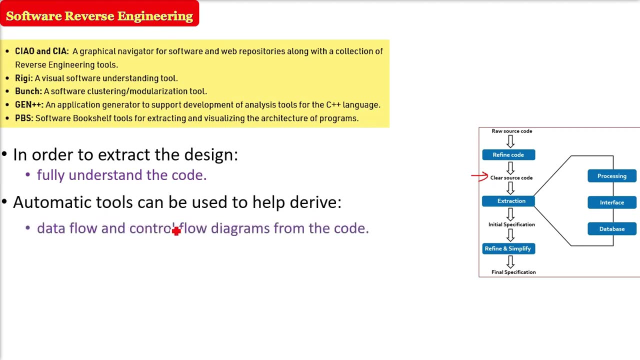 So in order to extract the design from the source code, you need to understand the code first. So there are certain automatic tools who can automate the process. It can give you from the code the data flow and the control flow diagrams from the code. 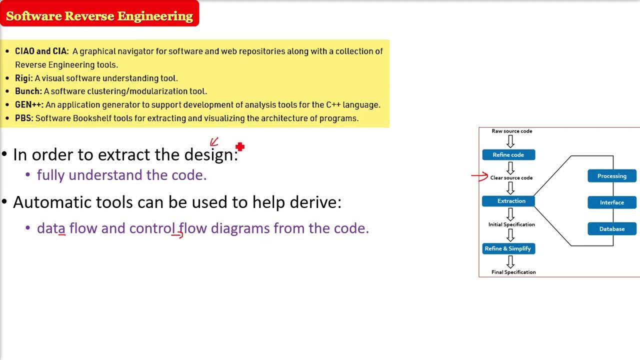 itself. So this is because the design would have lead to this code. So CIO, CIA, RIGI, BUNCH, GEN++, PBS, and there are so many in the market. There are so many. There are some open source also. 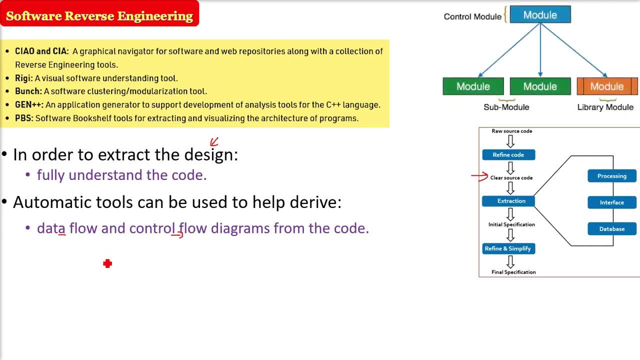 Some are proprietary. also, These automatic tools can be used. Then what you have to do? You have to extract or find out the structure chart. What is the main module, What are the sub modules, What are the library modules? So the module invocation sequence and the data interchange among the modules need to 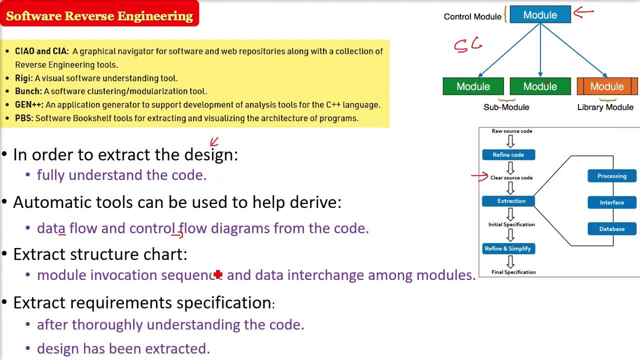 be extracted. And finally, when you have come up with the design, now you have to extract the specification, Because once you have understood the code, the design has been extracted. the next important task is to find out the requirement specification, and this requirement specification will be: 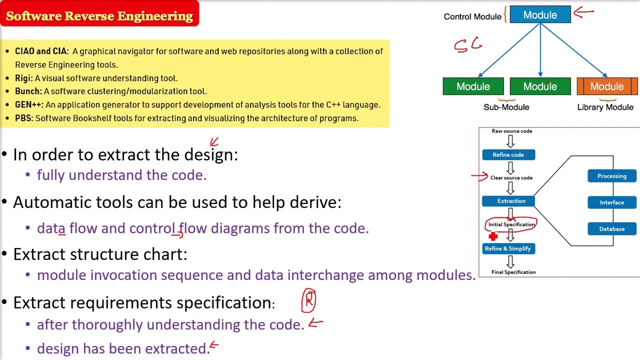 the basis for the forward engineering. Okay, so specification is the key, and they may not be that much true to what actually the old system might be having, But depending upon the design you have learned these are the specifications, So that's it, Thank you. 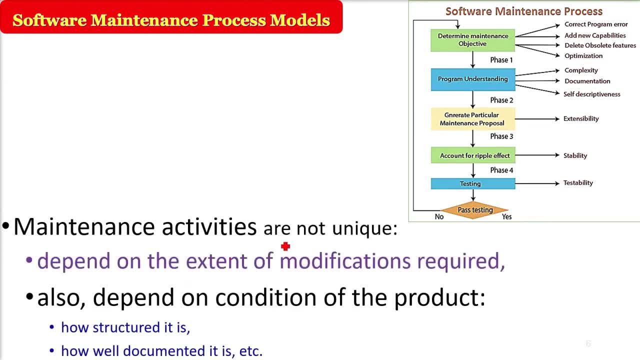 So software maintenance process models, maintenance activities are not unique for each and every kind of projects or software or system. It totally depends on what kind of what extent, of what complexity, of what way the modification request or change request is received. The modification will be different depending upon the different kind of projects under 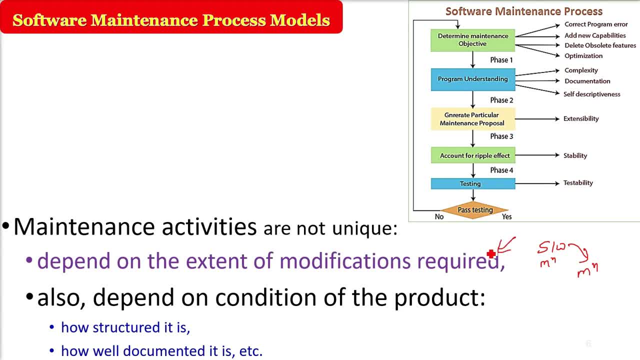 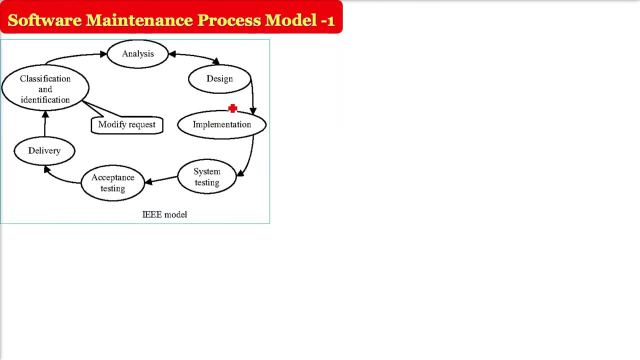 question. It also depends on the condition of the product, How well structured it is. Do we have the document or not? Do we have the proper say inbuilt documentation or not in the code and various supporting document? So we can have multiple software maintenance process models if the required changes are. 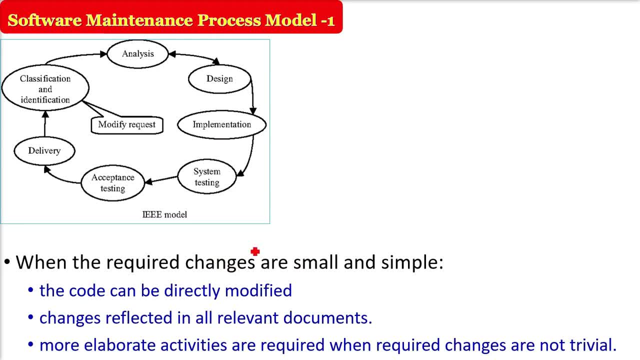 very small, meagre, they are quite simple and the project is also not very complex. then we can do one thing. We can directly go to the code and change it. This is called patch working or bug fixing. So these changes are reflected also to the relevant document. wherever you have to change. 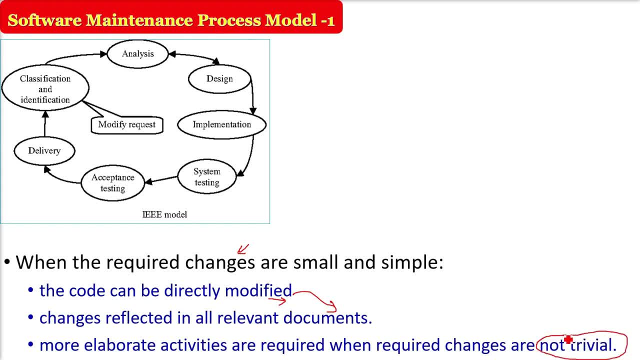 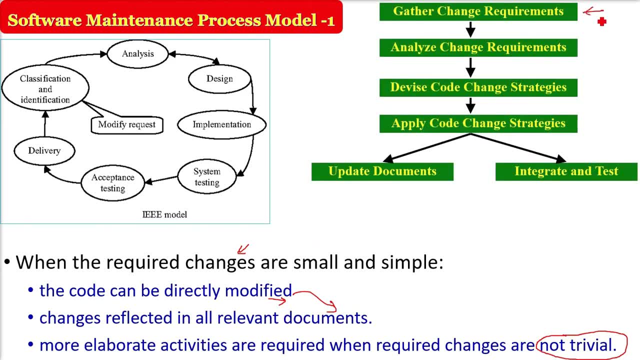 it And more elaborate activities are required when the type of project change. This is about gathering the change requirement. You need to analyze the change requirement and then what way you are going to change the code. You need to analyze and define the strategies. 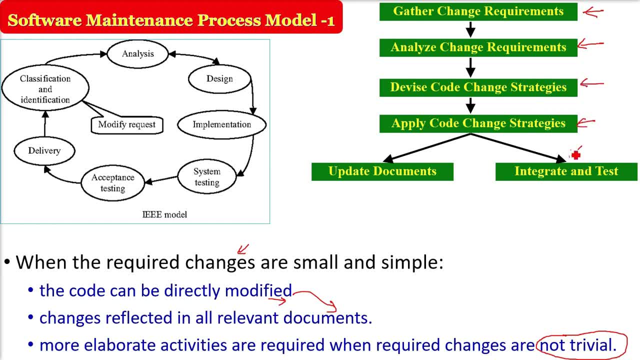 Then application of these code change strategies. Finally, the integration and testing and the relevant document updation should be done. Whatever you have done need to update in the present document. So IEEE model it is saying. then, once the modify request comes, you have to classify and identify. 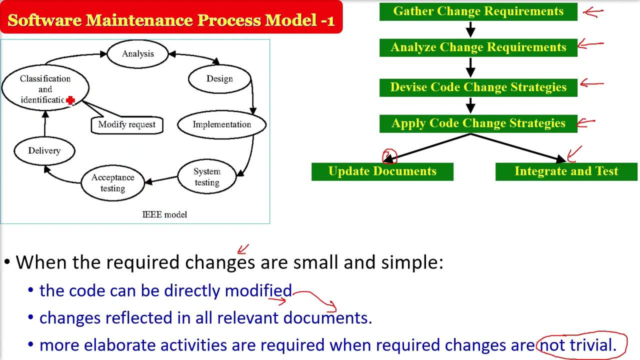 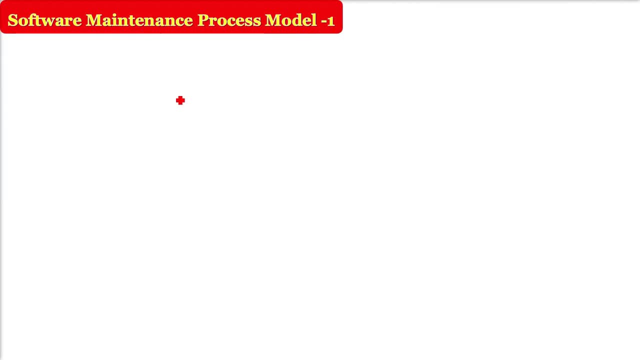 the modify request, Analyze the modification where it has to be done, Do the designing: Implement. the design Implement, do the testing again and then the acceptance testing by the user, and then you deliver. So this is how the circle will go on in the maintenance activity. 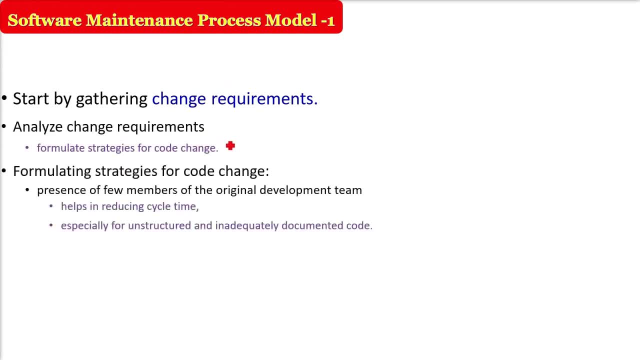 So first we will start by the change requirements gathering. We have to analyze the change requirement. that is how to change the code. You have to formulate the strategies. You cannot just go to the code and change it And then see if the original development team member is present. 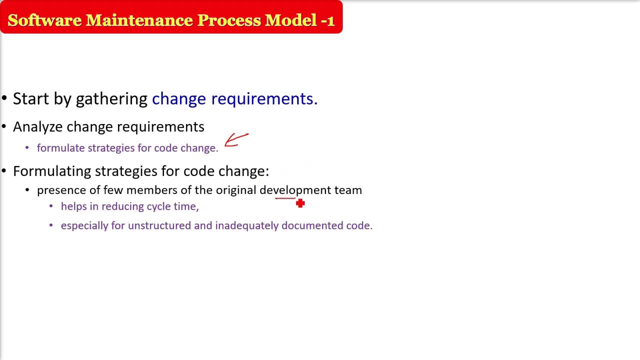 If the original development team member is present. If the original development team member is present, How to formulate strategies for code change? If the original development team member is there, it will reduce the working time and specially when the code is very unstructured and you don't have the documentation properly. 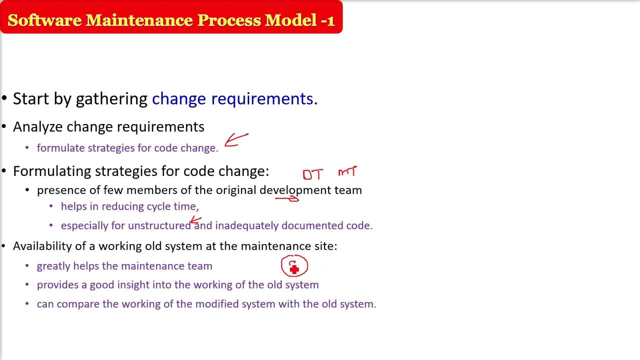 Also, if you have the old system available with you, that is the old system now as a maintenance engineer, it greatly helps you because it gives you the insight of the old system working old system. Now when you modify the system, you have the comparison. okay, I use. this is my modified. 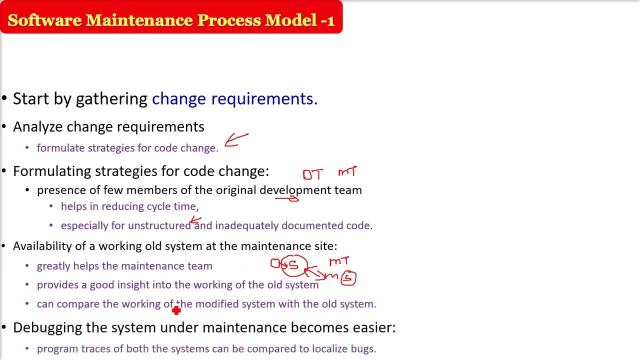 system. this was the old system, this is what we have changed, And also both systems are in front of you so when you are debugging, program traces of both the system now can be compared so that you can localize the bugs and fix the bugs. So this is the. you know if you have the team team, earlier team and earlier system. 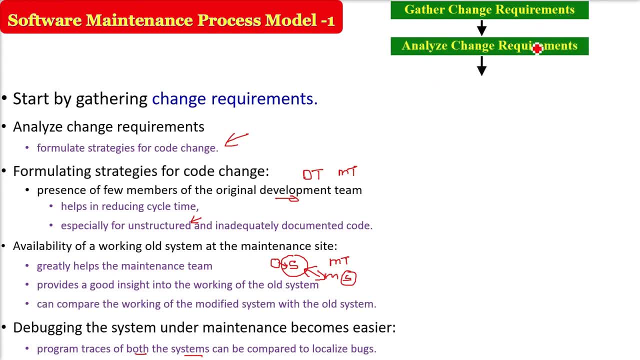 So you need to gather the change requirements. So this is the you know. if you have the team team- earlier team and earlier system, So you need to gather the change requirements. So this is the you know. if you have the team team- earlier team and earlier system. 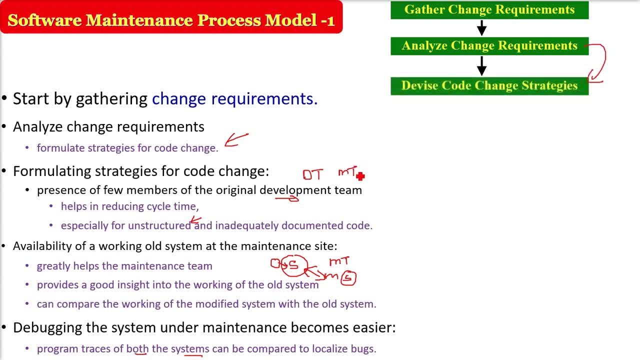 So you need to gather the change requirements, Analyze the change requirements, devise the code change strategies and, as I said, you have to implement the code change strategies. application of this and, finally, testing and the documentation application. So this is the software maintenance process model number one. 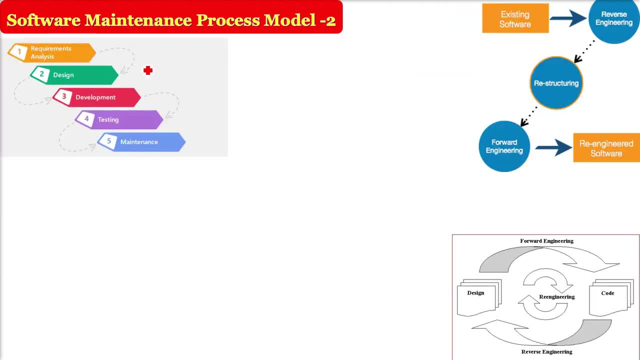 There can be multiples software maintenance process models. So this model- if the software is a complex software and the complex maintenance projects are there, So we need to apply this software re-engineering. okay, because the amount cost to replace the software is very high. So we need to start with the reverse engineering cycle and a forward engineering cycle, both. 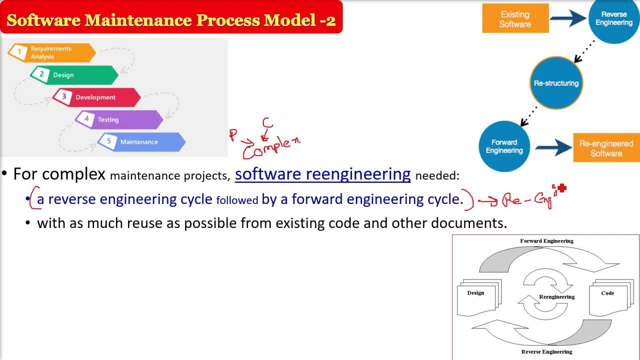 are combined and called as re-engineering. So forward engineering plus reverse engineering is nothing but the re-engineering. And here we will use or reuse, you can say- the existing code and the documents. so if you want to, you know run or high jump, long jump or high jump, then you take step back. 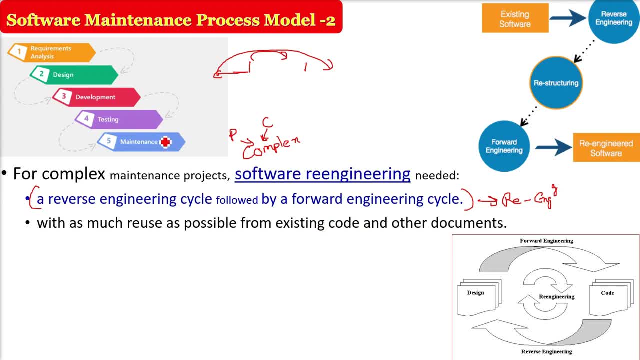 and then you jump. So when you take step back, that is the reverse engineering. then you jump forward, that is the forward engineering. So you are going from maintenance to the development code, code to design, code design to requirement analysis. So finally, you are trying to find out the requirement specification. then you combine, 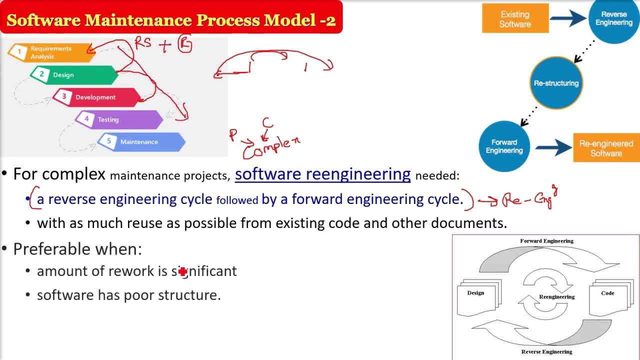 this with the present requirements and then you go with the SDLCs, whichever you want to follow. So this kind of software maintenance process models are preferable when amount of rework is quite significant and software has a poor structure. So the rework if it is significant. we cannot just go and do the patchwork or fix the bug. 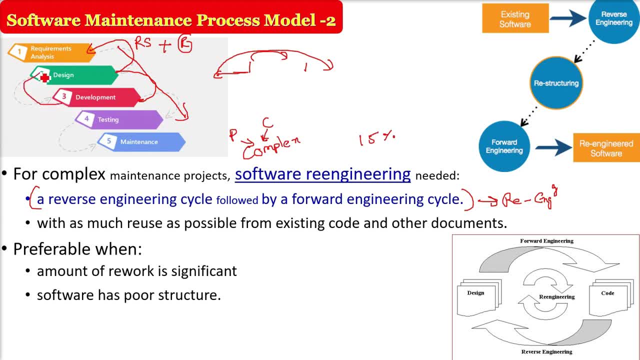 at local point. We need to reverse engineer and then find out the specification and then only with the new specification do the proper, the application of software engineering principles. So that is called the forward engineering cycle. Forward engineering cycle comes only after the reverse engineering cycle. okay, 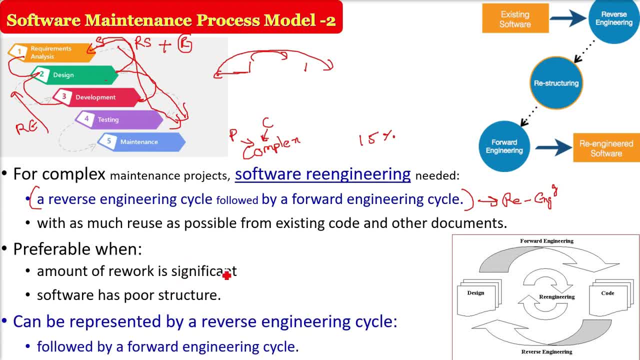 So this can be represented by a reverse engineering cycle. As I said, reverse engineering cycle always is giving rise to a forward engineering cycle. There is no separate forward engineering cycle. So this is the existing software. First you will start with the code going to design, then to the requirement specification. 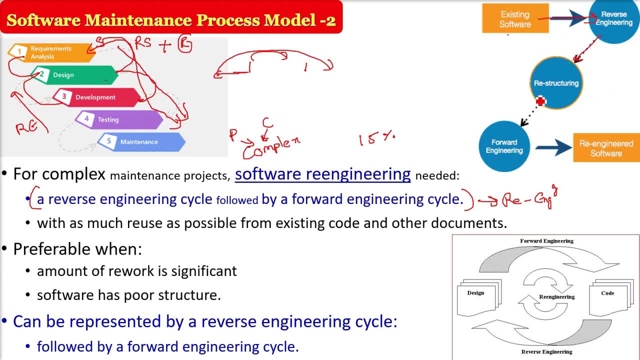 and then you will restructure, And then when you restructure you go to the forward engineering and then you produce the product called re-engineered software. Here also you see that code to design and design to code. First you have to start with code, go to design, that is reverse engineering, then again from 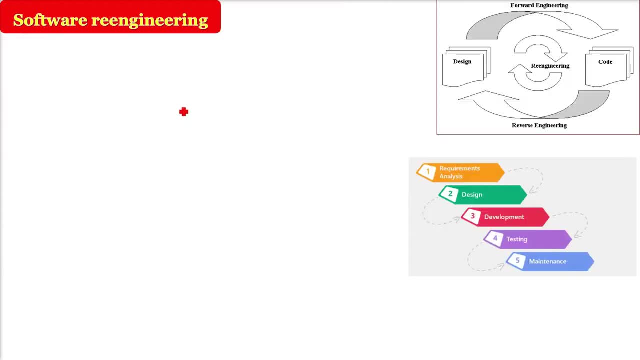 design to code. that is the forward engineering. This whole process is re-engineering. So software engineering re-engineering because many of the software products they need a lot of maintenance. They are aging software. You are starting from code, you are going to design, design you are going to requirement. 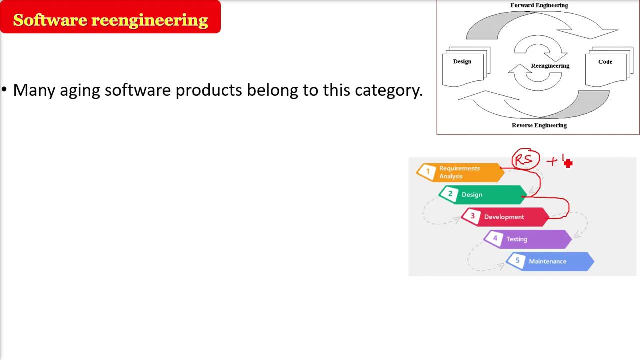 specification. Now you are adding the new requirements or the change request and then you are going again forward from requirement specification till the testing process that is called the forward engineering. So reverse engineering plus the forward engineering is called as the proper re-engineering. So during this reverse engineering the old code is analyzed. 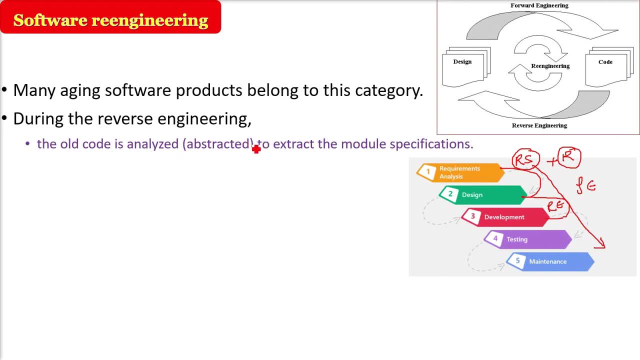 That is, to every level of abstraction, because we need to find out the or extract the module specifications. Now, when you know the module, how is the cohesion coupling, how is the module being formed, what is the patterns you have used and what are the architecture? 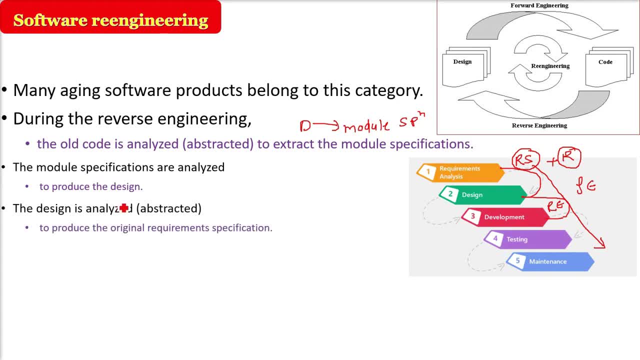 The module specification are analyzed in order to produce the design. and then the design is analyzed: That- what requirement, what use cases has finally devised this design, has created this design. And then you come to the original requirements. So what is the original requirements? 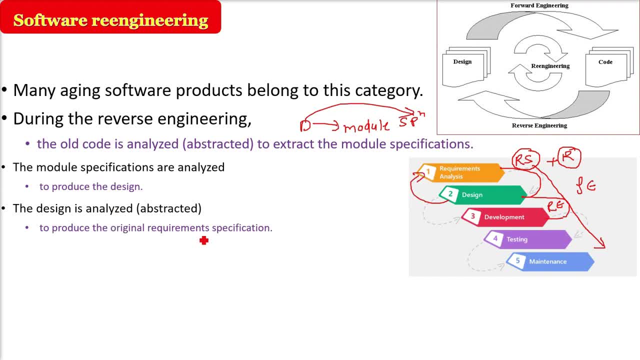 So once you have the original requirement specification which has come from design, which has come from the old code, Now you add this with the change request. Now the change request or change proposals are then combined with the requirement specification. Now you arrive at the new requirement specification. 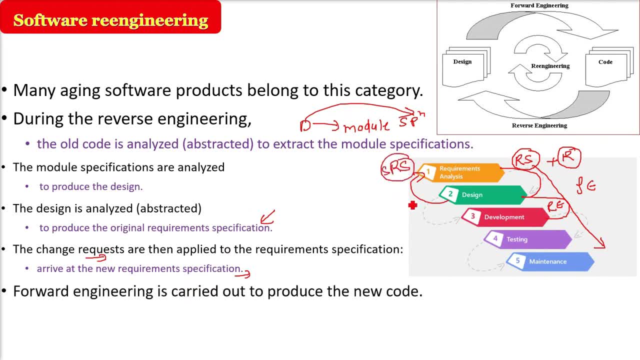 Once you are having the requirement specification, it is just like creating a new software. So now you do the forward engineering to produce a new code and during this, during the design modification, There is a substantial reuse because there are reverse engineer products we can use. 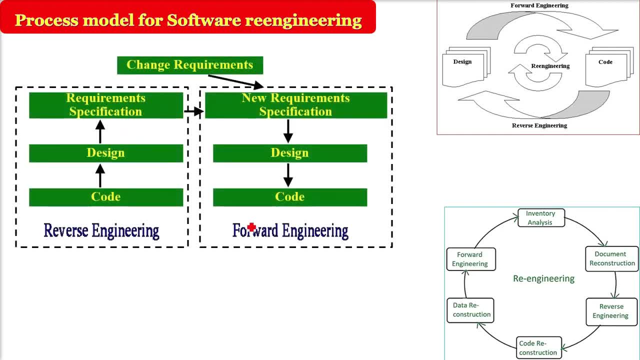 Process models for software re-engineering, because whenever you have a big project and big proposals to change, you start with the reverse engineering. You already have a code with you and there can be document to support, to help you, or there may not be.